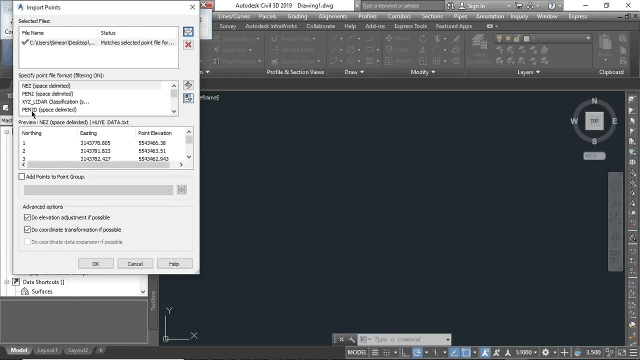 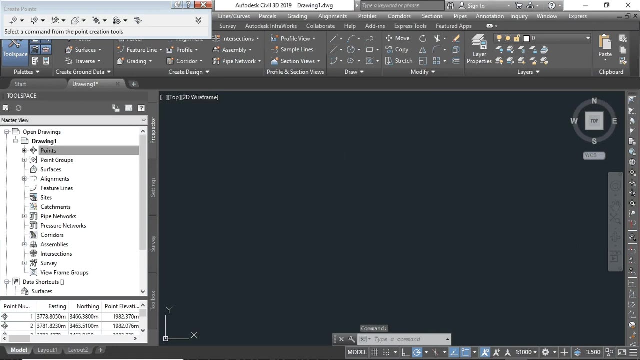 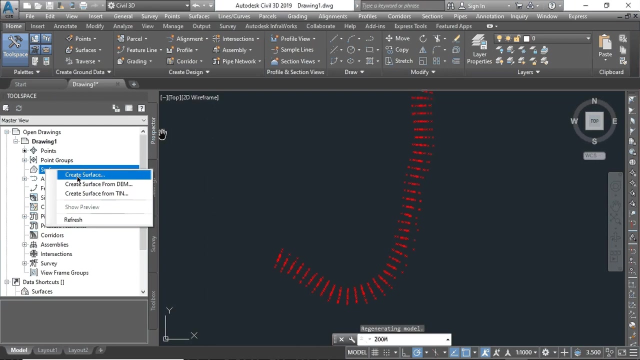 we have no nothing. you click on pnz- space delimited- to get this nothing. so then you click: okay, yeah, you come to the window and right click, then you zoom, right click again, then zoom, extend. as you see, this is our data up. after importing our data, we, we create our surface. come to surface, right click, then create a surface. 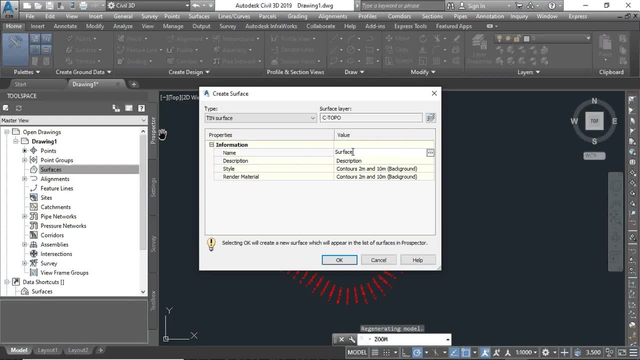 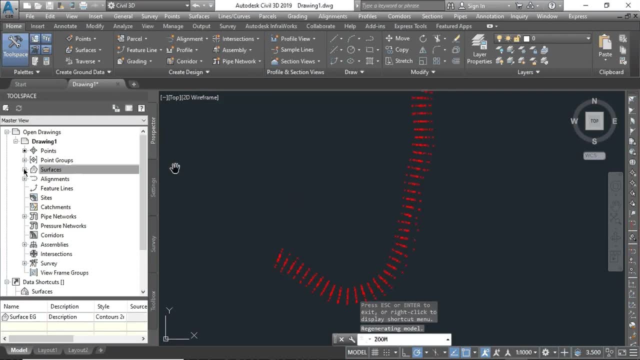 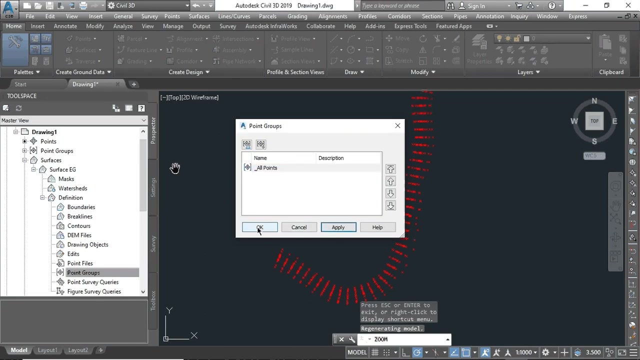 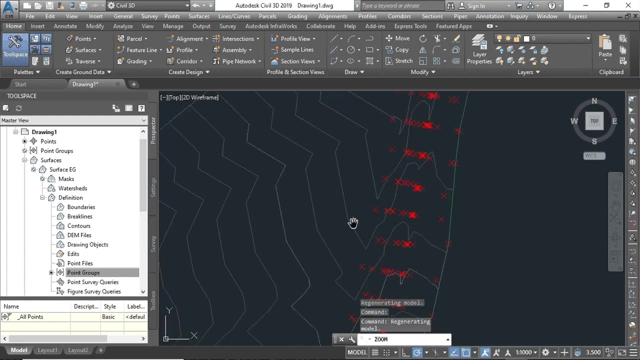 then let's call it surface eg. and okay, you come to surface this positive sign, then the surface you have created and the click on definition, then you come to like the click on point from group, then you add: click on all point you apply, then okay, as you see, this is our surface we have created. after creating our surface, we go to center line. 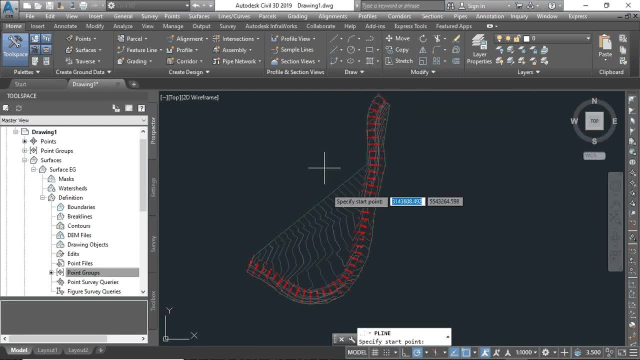 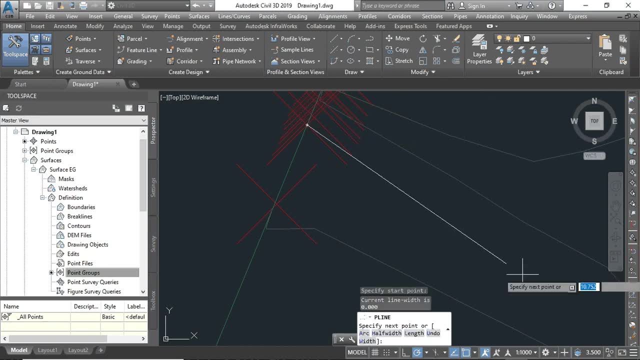 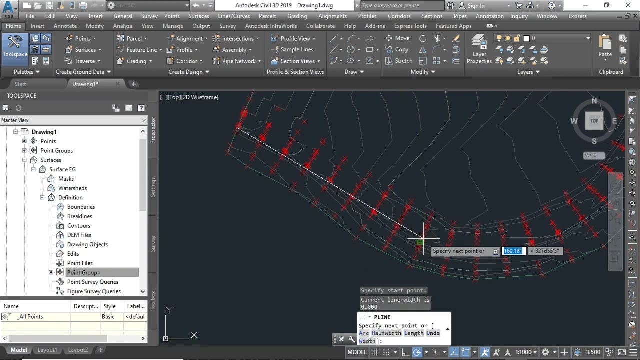 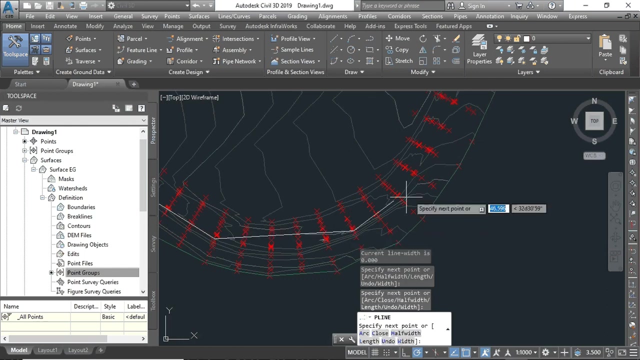 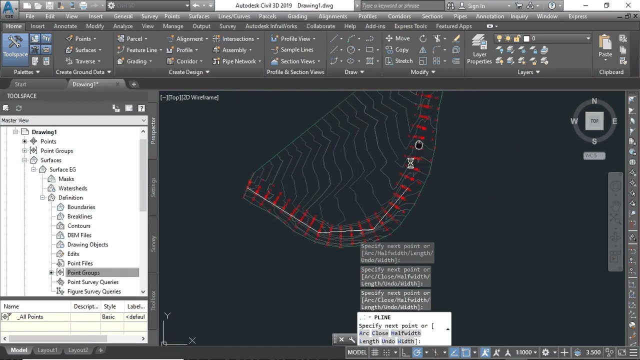 centrine. you click on polyline symbol. then you come to draw your center line. remember this: this is centrao. it will help us to get this center line. we have to get this center line width of the load. it should be used as reference to get all parts of the load. 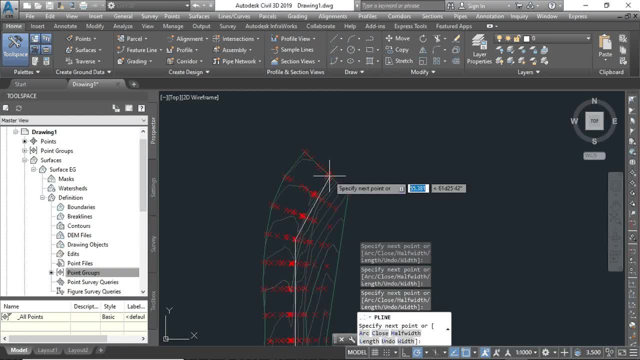 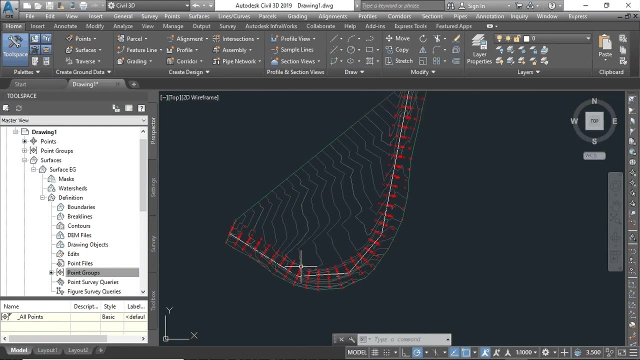 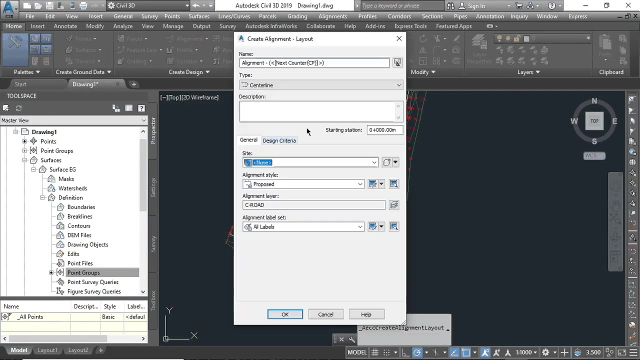 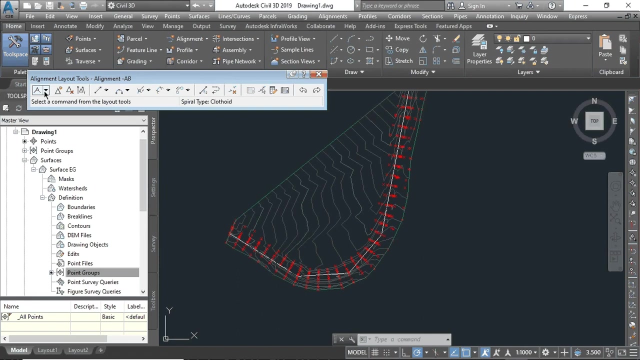 then right click and enter. as you see, we have finished to draw our center line. after drawing our center line, you click on alignment, then alignment creation tool. let give the name of alignment. call it a b, alignment a b. okay, you see the toolbar. they give us alignment. 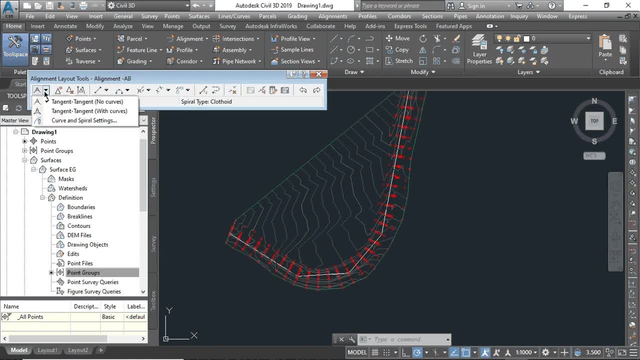 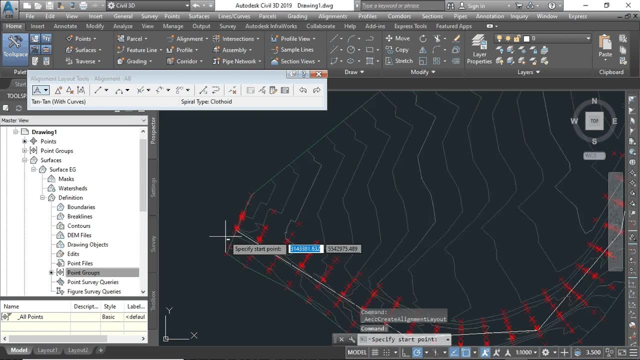 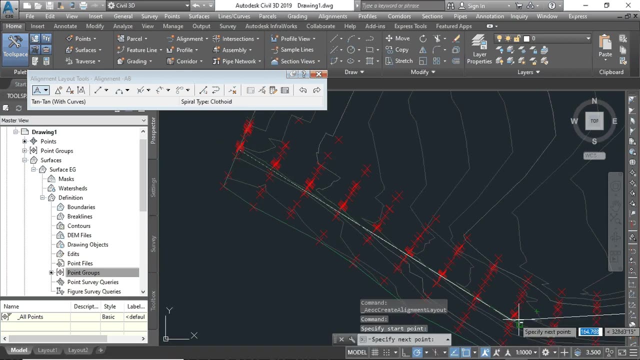 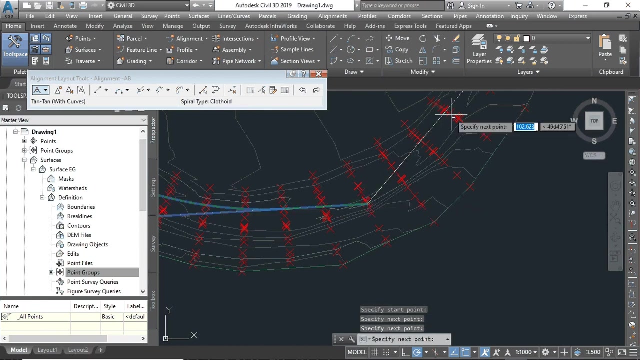 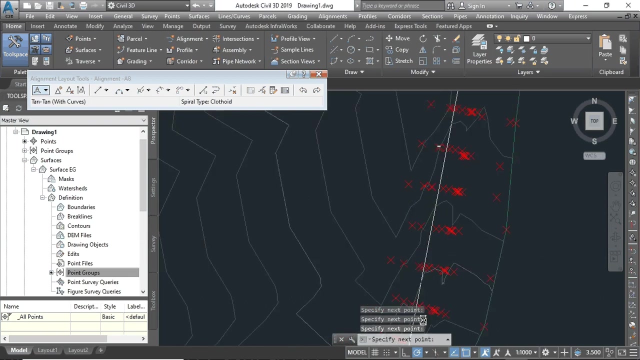 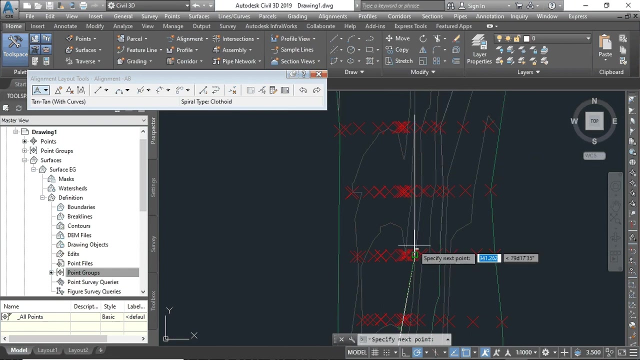 layout tool. then you click on this symbol, then choose tangent with curve. here we are going to make the horizontal curves. this is horizontal alignment. as you have seen on the last sessions, we are still making our alignment. it is better to make alignment by following the the center line. 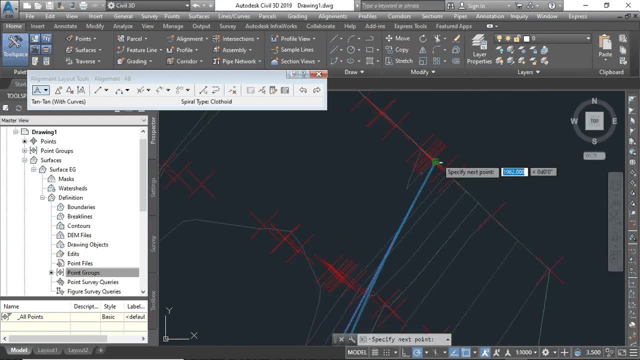 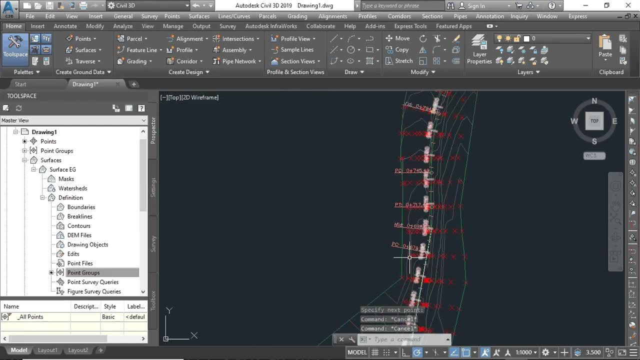 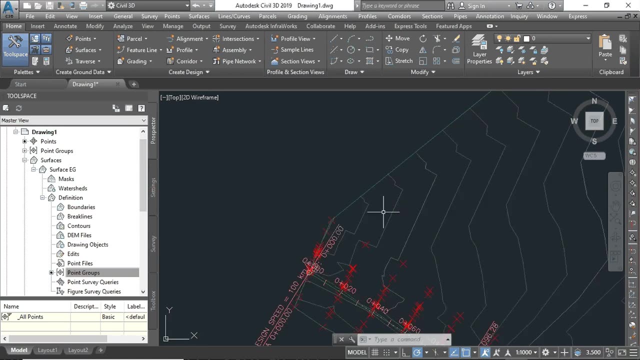 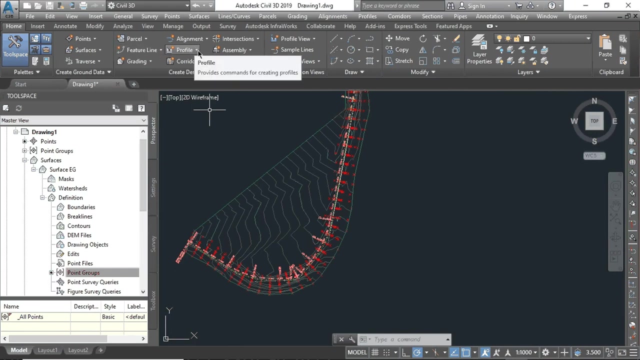 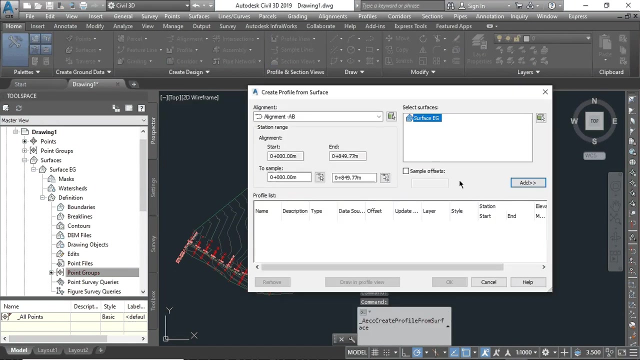 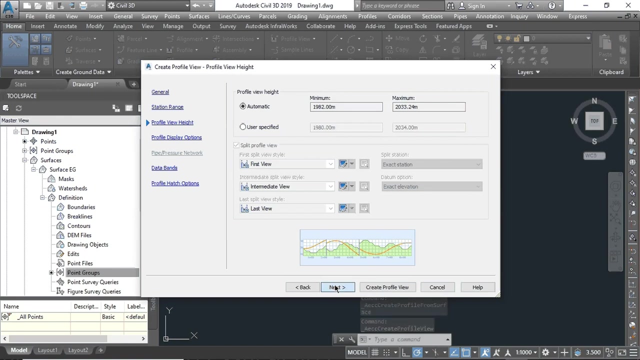 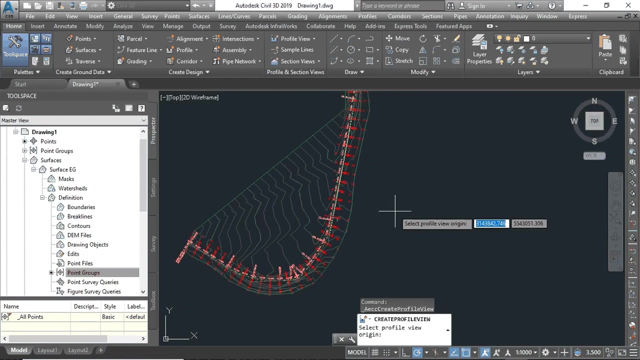 then you click, right click. as you see, this is our alignment, this is our align니ment. after creating horizontal alignment, we go to profile: click on profile created suffers profile. then you add, then you click on draw in profile, then next, next, click, next, then you get a profile view. you click anywhere in the 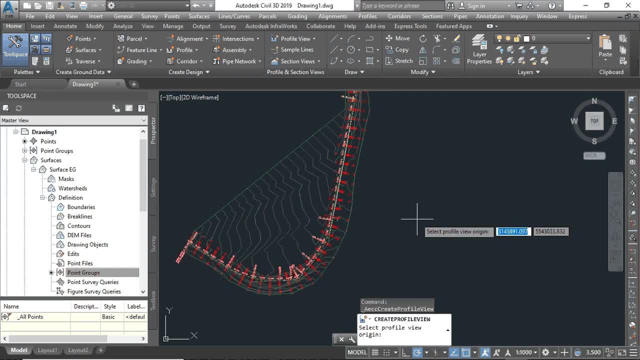 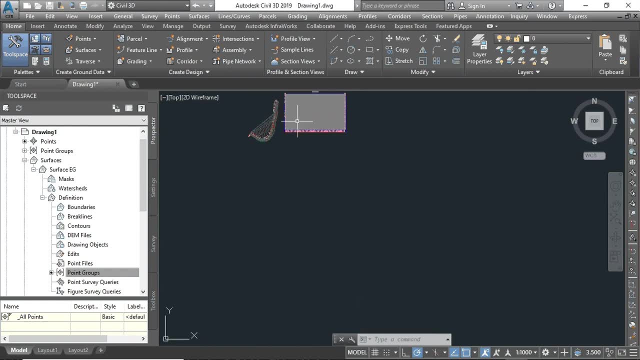 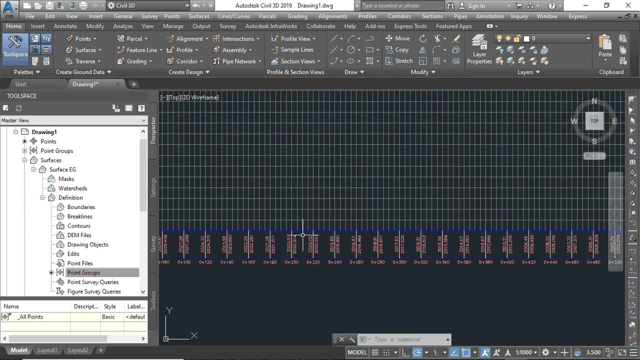 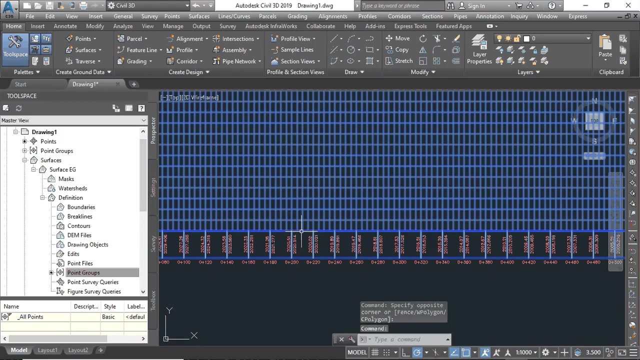 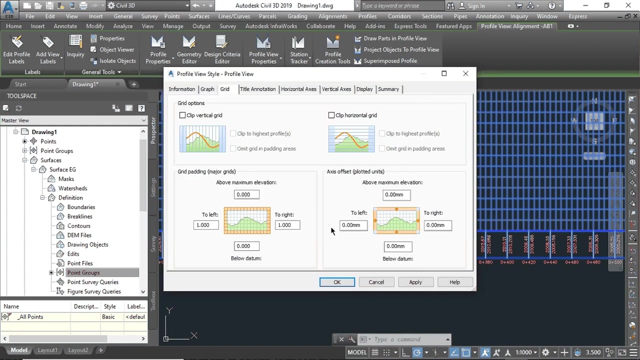 drawing in the window. so this is our profile. as you see, this is our profile. so let us edit our profile to still have only the terrain. you select the profile, right click, you edit profile view style. then you come to grid. you click vertical grid and horizontal grid. 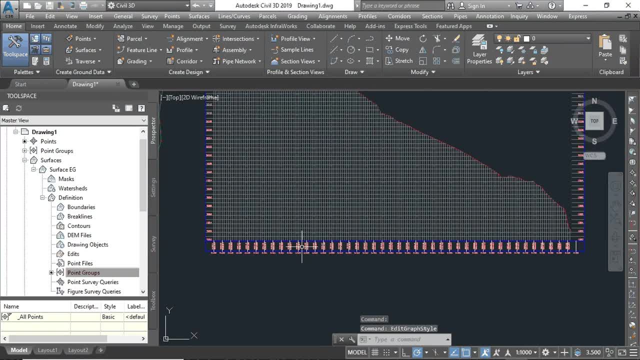 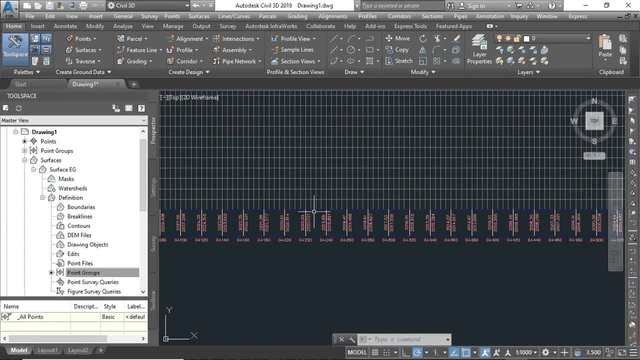 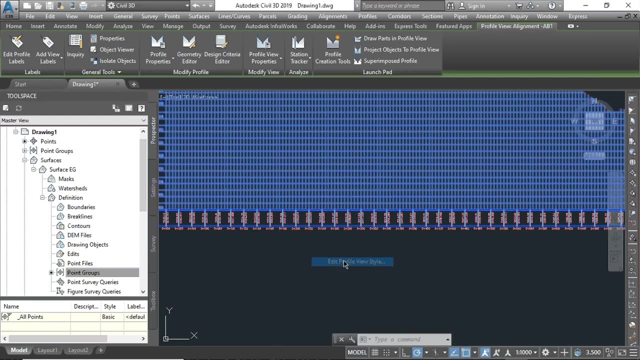 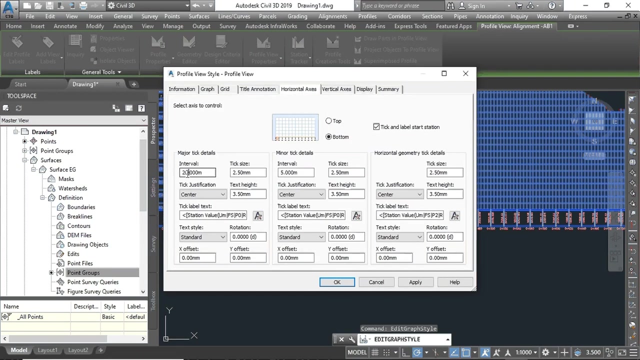 you edit profile view style. then you come to grid. you click vertical grid and horizontal grid, then you apply. so, as you see, you can also edit the. you can also edit the interval. you select your profile, edit profile of your style again, then you click on horizontal axis on the interval. let us choose 25. 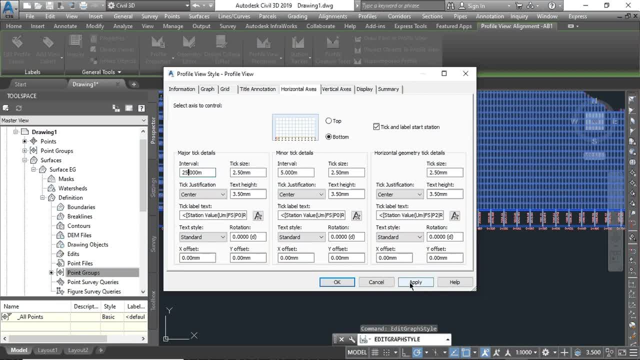 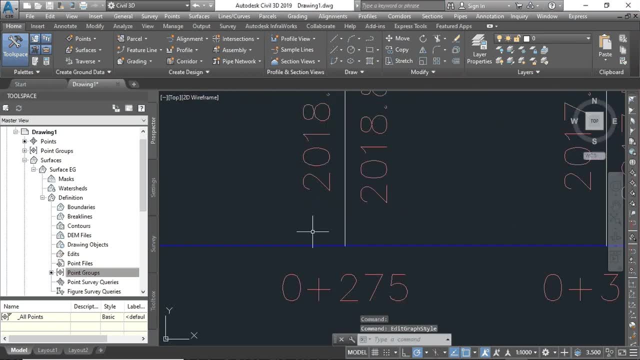 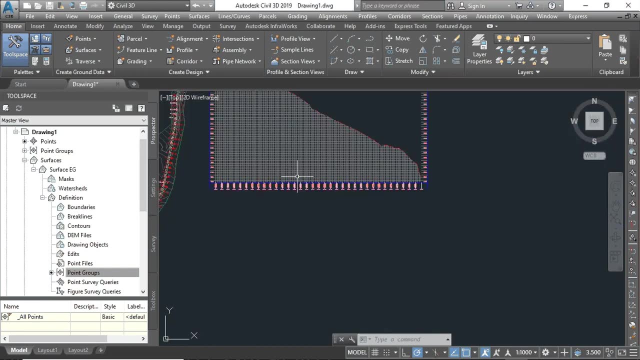 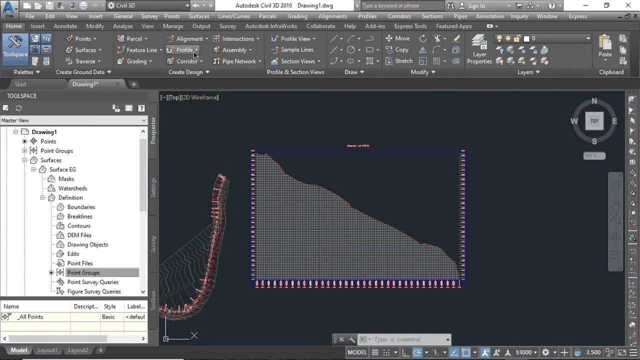 close that to have interval of 25. then you apply this is a horizontal interval that we, as you see, we we edited even the vertical. you can can do so. after that, we are going to make a vertical alignment. you come back to profile then profile creation. profile then profile creation. 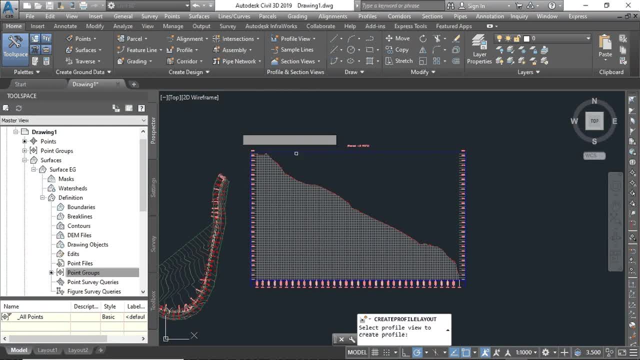 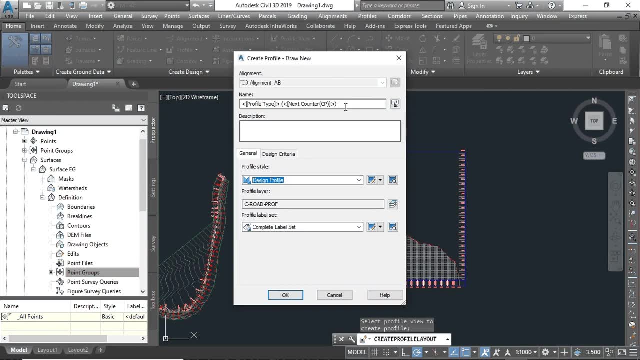 profile, then profile creation tool. you see this symbol. you click tool. you see this symbol. you click tool. you see this symbol. you click anywhere on the drawing, then you give anywhere on the drawing. then you give anywhere on the drawing, then you give the name, profile name. let us call it. 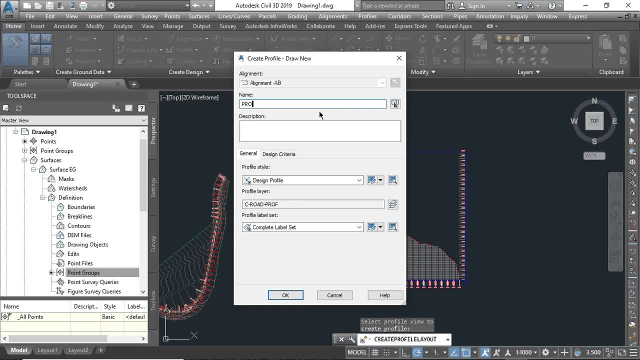 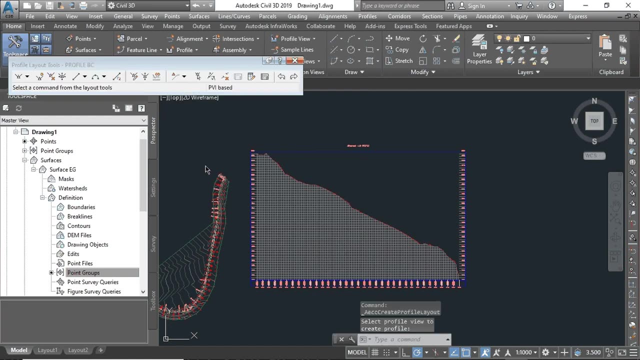 the name profile name. let us call it the name profile name. let us call it profile profile profile. profile profile profile BC, BC, BC, BC. okay, okay, okay. you see this toolbar profile layout tool. you see this toolbar profile layout tool. you see this toolbar profile layout tool. you select time, draw tangent with curve. 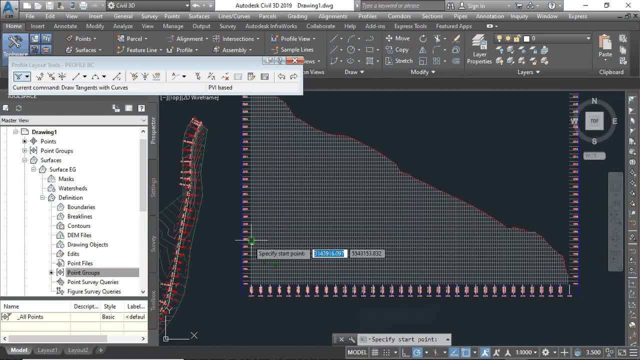 you select time: draw tangent with curve. you select time, draw tangent with curve. so we are going to make our. so we are going to make our. so we are going to make our vertical curves vertical curves. so, as you see, this is our, our vertical. so, as you see, this is our, our vertical. 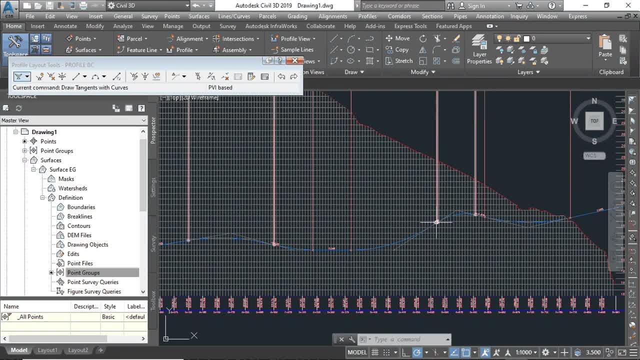 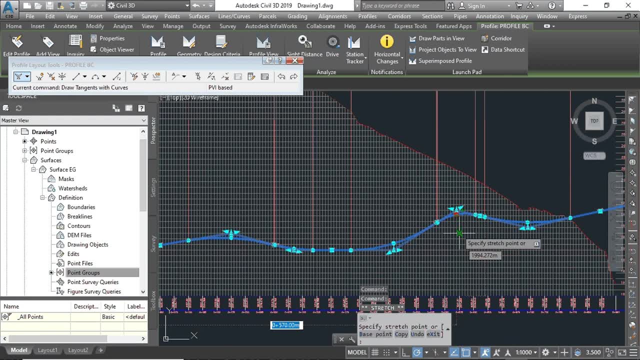 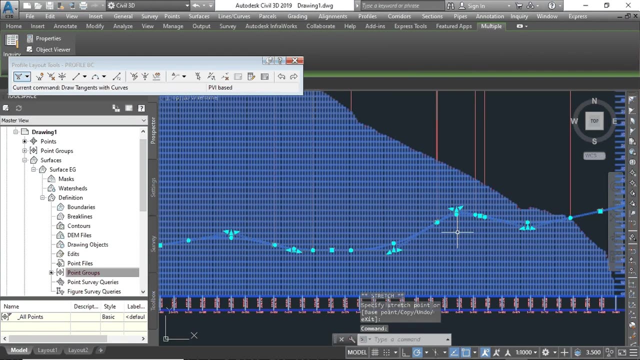 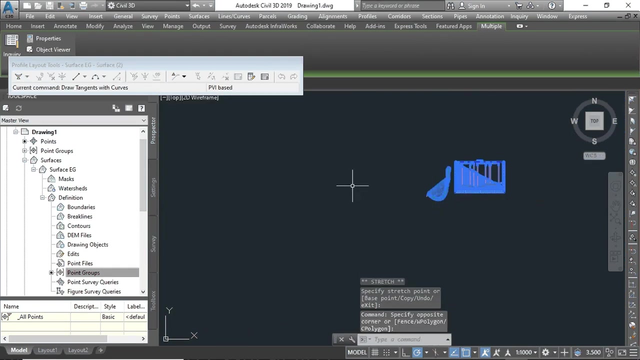 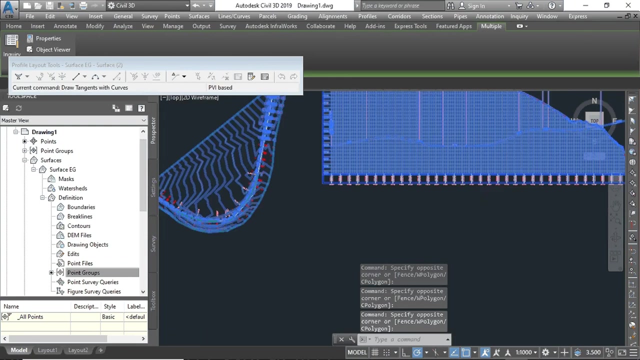 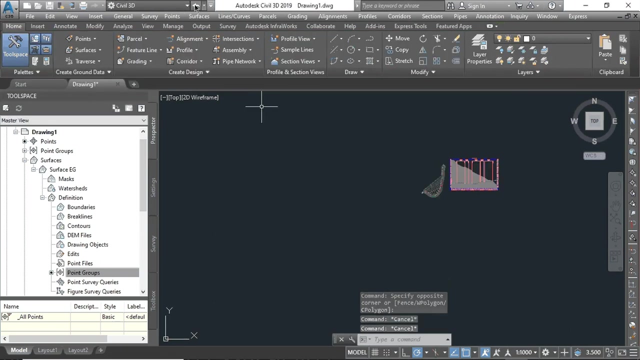 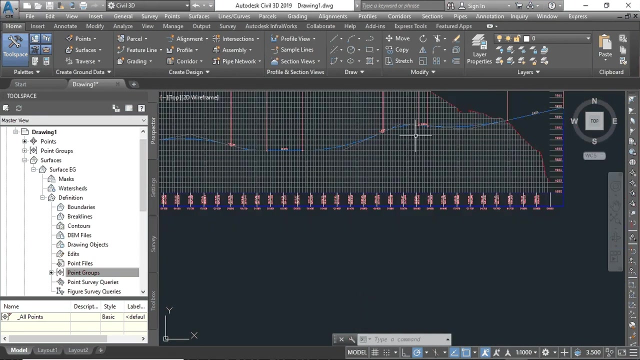 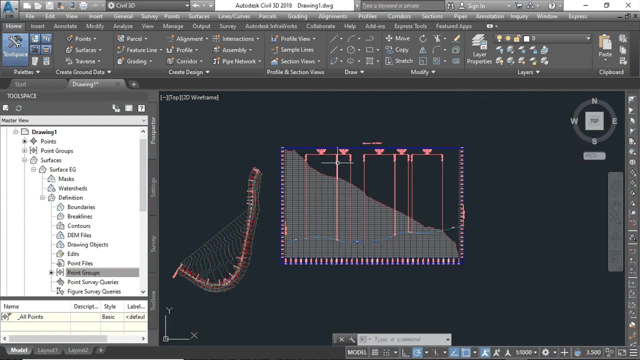 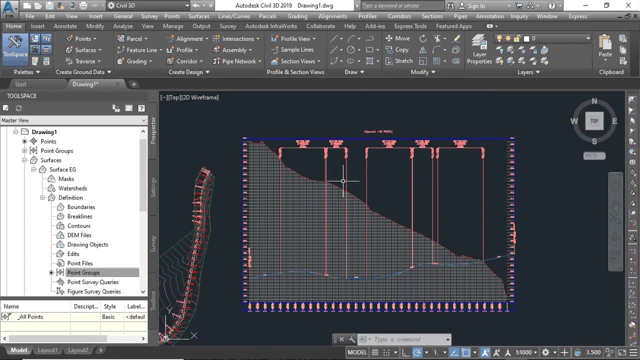 so, as you see, this is our, our vertical curves, vertical curves, vertical curves. so, as you see, we have vertical curves with vertical lines and vertical lines, Thank you. So this is our vertical curve. After that, after creating the profile, we create our assembly. 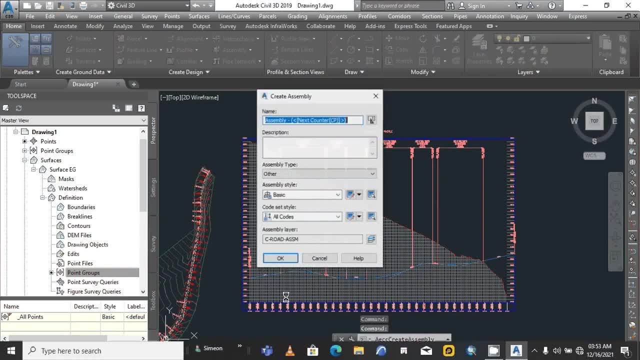 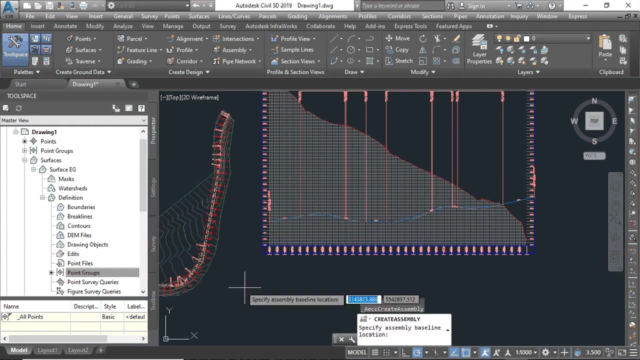 We click on assembly- create assembly. then we give assembly name the name. let's call it assembly AC. Then, okay, We click anywhere where we want to display our assembly. As you see, we have our assembly, Okay. 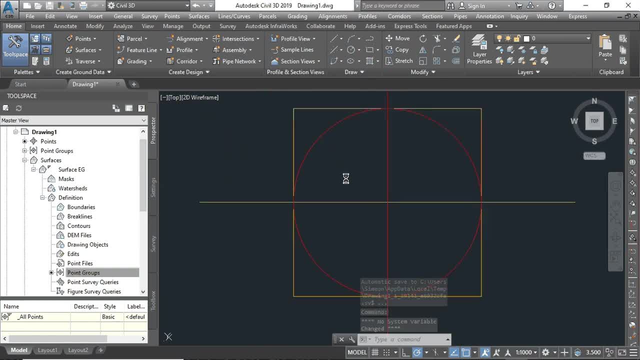 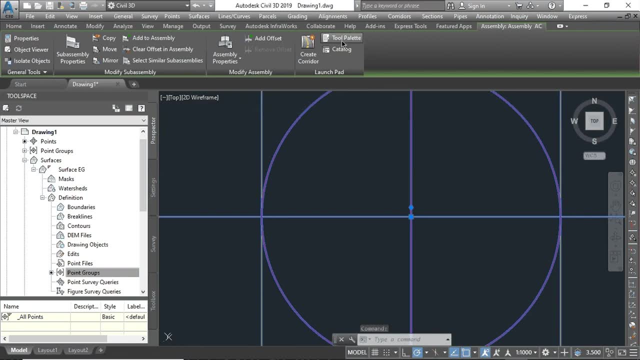 As you see, this is our assembly. You click in the center, then you see some tool palette. you click on it, You see basic rain. Every part of the road is there. Let us start by rain. We choose rain, We choose rain. 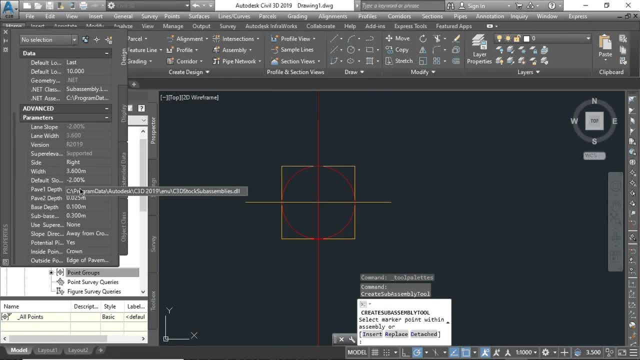 Okay, So this is our activity. We choose rain, We choose rain, We choose rain, So we add it. Our task is to use three as width, Then sub-base, we have task to use 50.. Then base: we are supposed to use 0.4 meter. 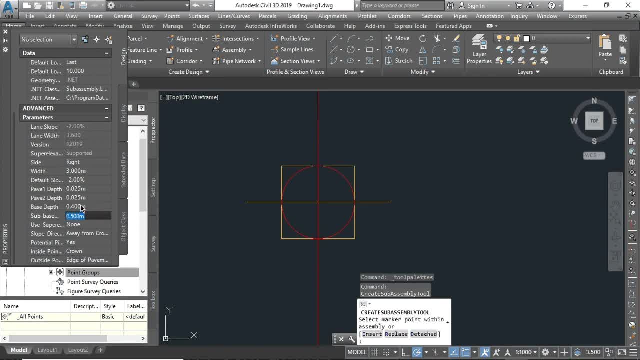 Okay, So we addé 30,0,5.. 0.15 on Pavement 2 and 0.1 on Pavement 1, so default slope, we are supposed to use 2% then. as you see, we are on the light. 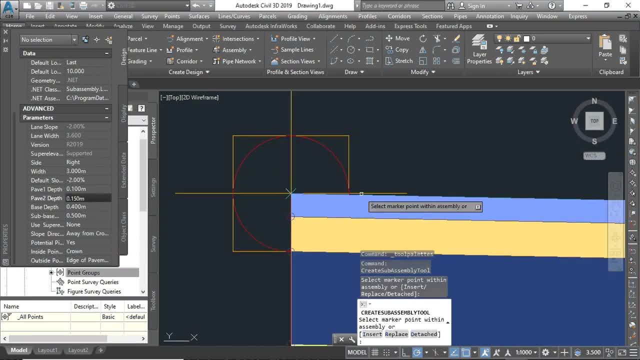 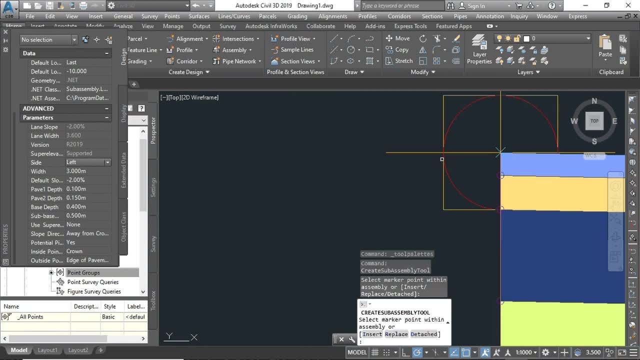 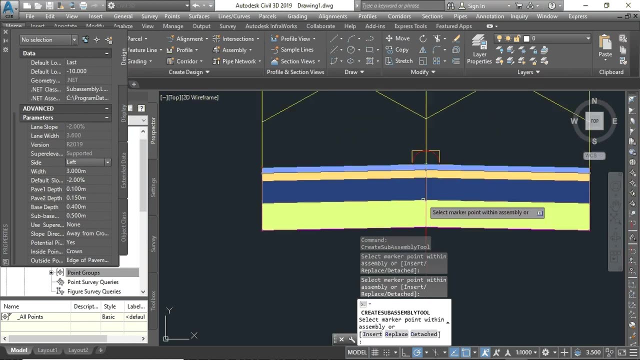 we are going to display it on the light. then we come back and choose left. after that, as you see, this is our end. then we go to shoulders, so I supposed to use the the we are supposed to use 1.5 in width, so other layers I supposed to use by default. 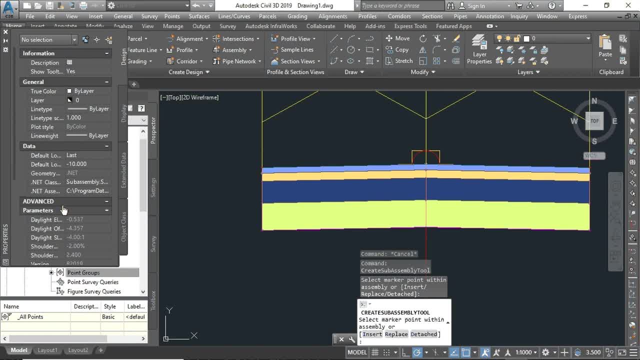 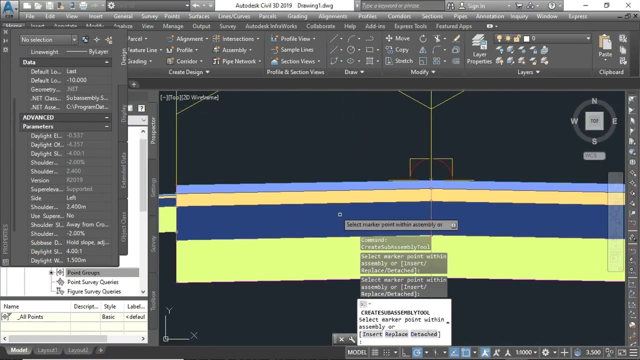 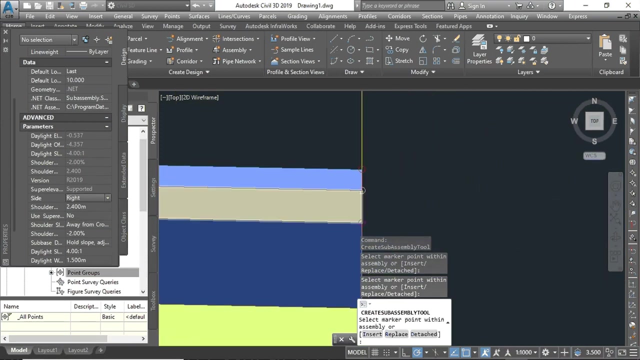 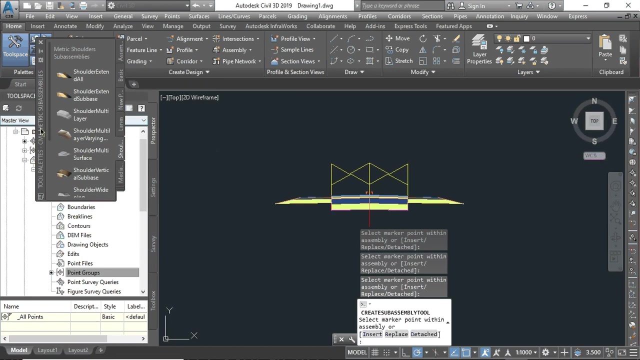 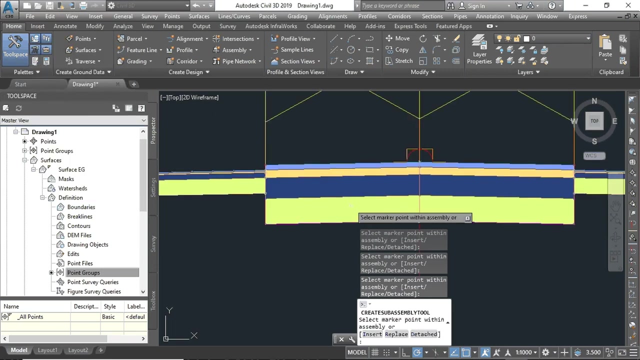 so, as you see, we are on the left- this is our shoulder- and go to the right. you click on the right side to get our shoulder. after getting our shoulder, we have to get some. we have to get some gutters. we have to get some gutters. 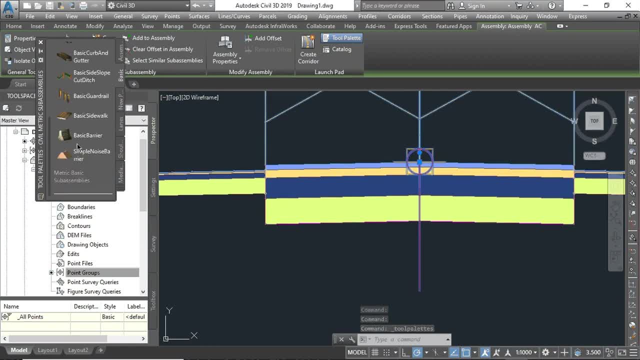 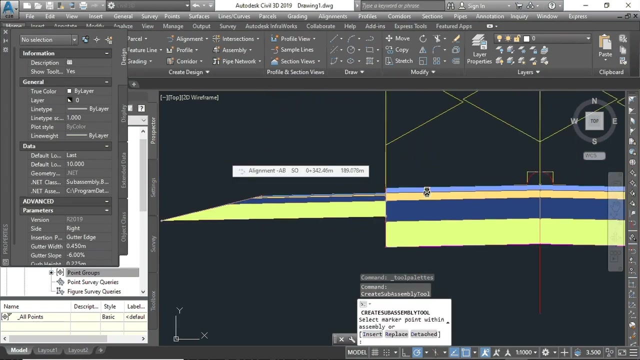 let us use some gutters. I supposed to use some gutters between shoulder and basic sidework. I supposed to use some gutters between shoulder and basic sidework according to my design. if it is innovation or if it is a mistake, I am waiting for my lecture feedback. 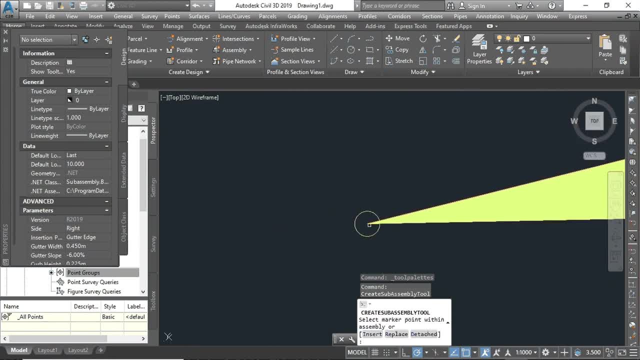 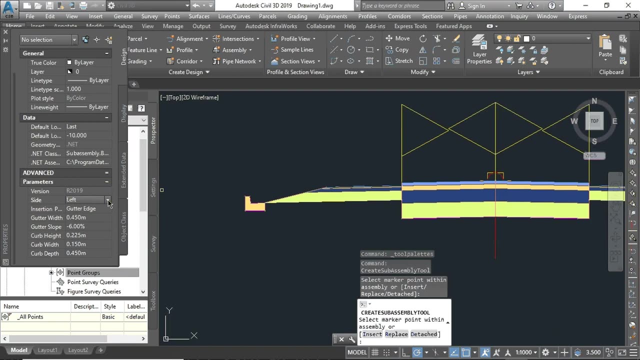 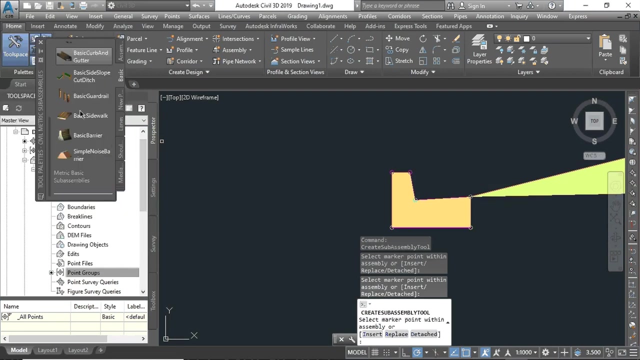 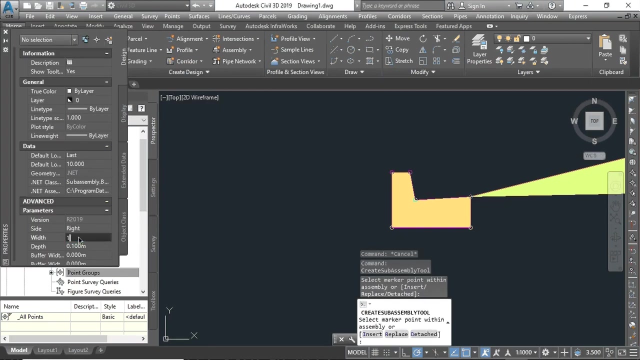 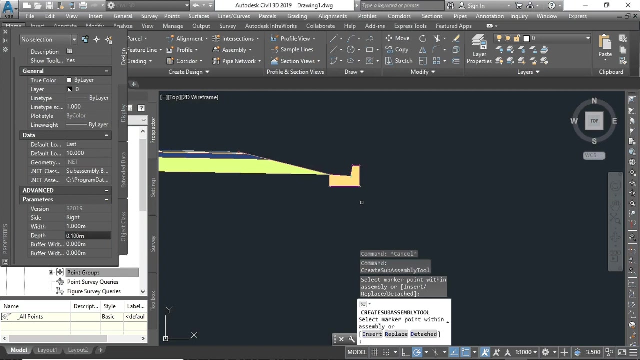 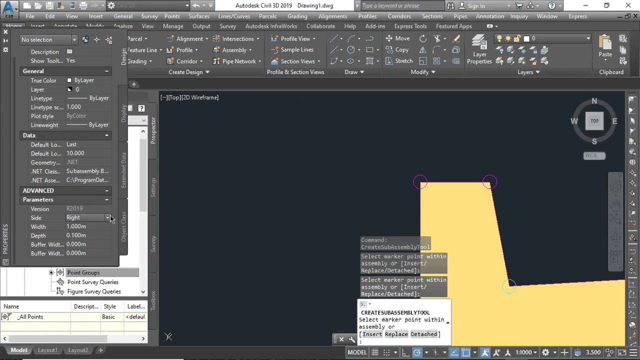 I am waiting for my lecture feedback. I am waiting for my lecture feedback. you can see that the, you can see that the and straight, and Then go to the basic side work we edit. let's make one meter to the light, Turn to the left. we are turning to the left. after that, I suppose to put some, we are. 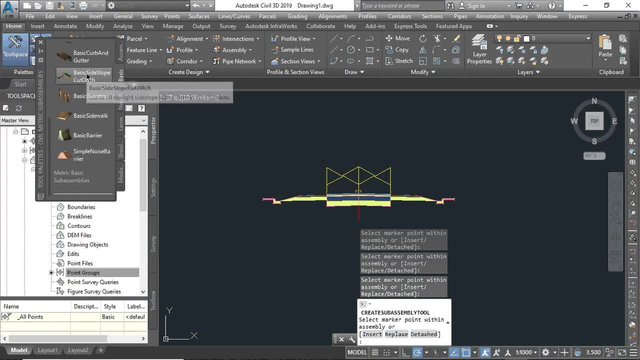 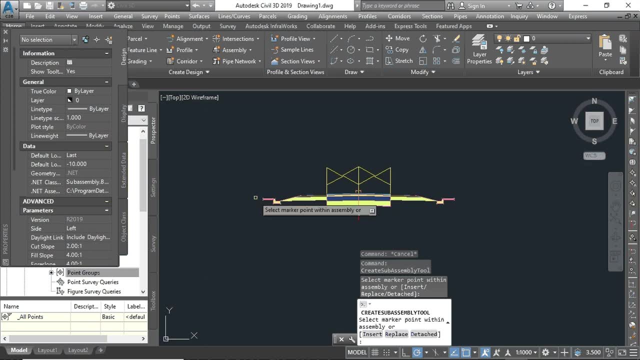 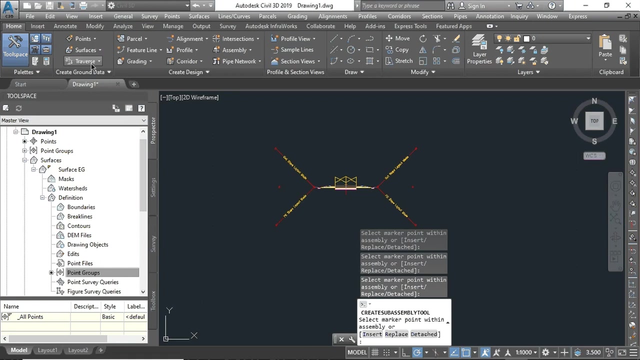 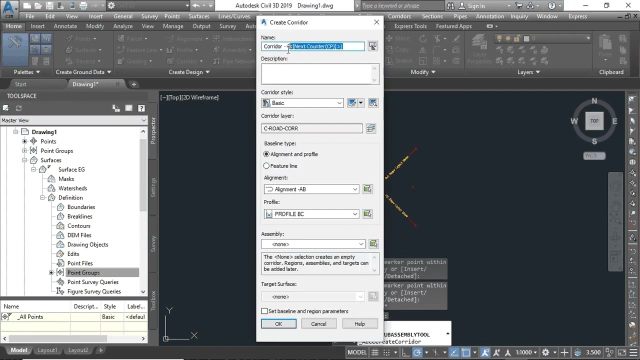 going to use some basic side cut slope, Dutch slope. So we are on the left and go to the light. As you see, this is my assembly. After creating our assembly, Uh, We create a profile. uh, I'm sorry, we create corridors. click on corridor, then we edit. 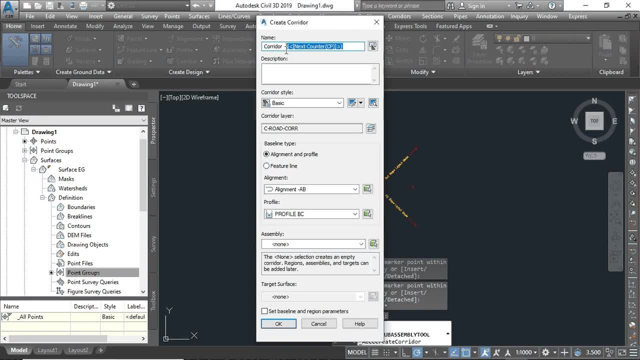 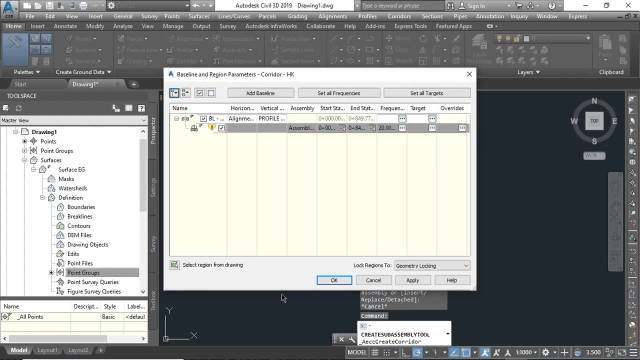 the name. let us call it corridor gg and let us call it corridor hk. Then we select: our alignment is a- b, our profile is b- c, then our assembly is a- c, then our surface is selected, then okay. 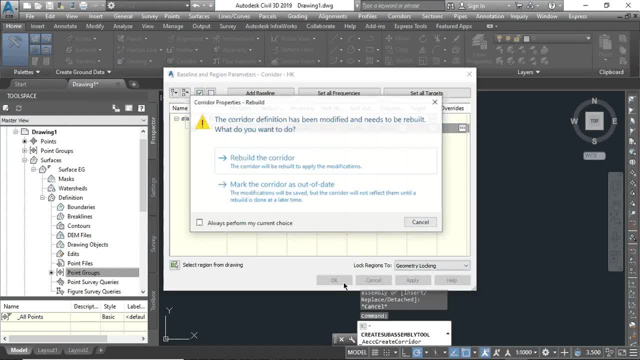 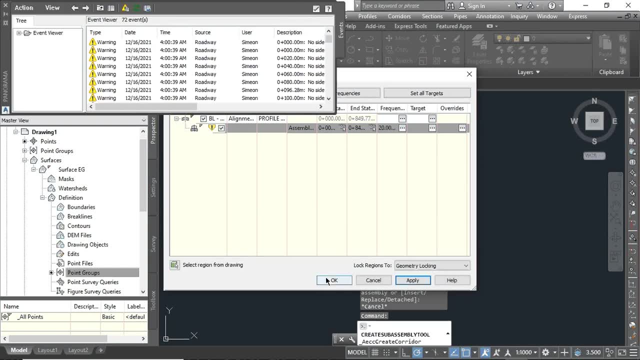 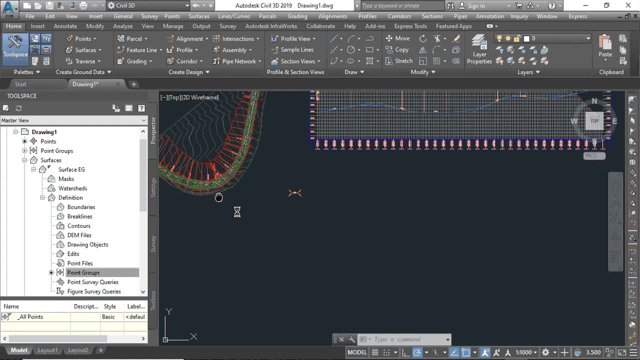 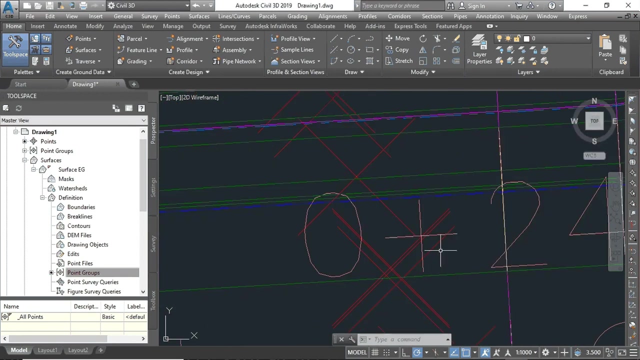 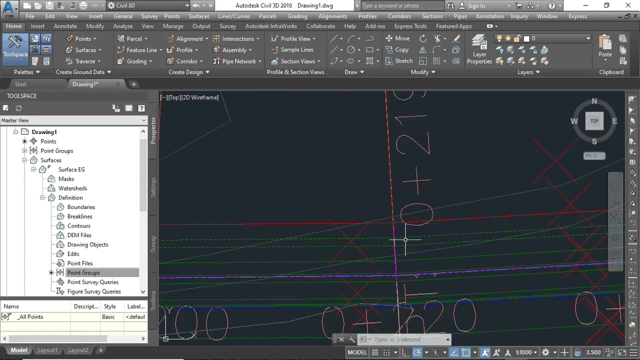 After that we apply, Then rebuild the code And we have our corridor: Click. okay, As you see, this is my corridor. So you select, we click on this thick light, Then you write click. I think I have done it fine. 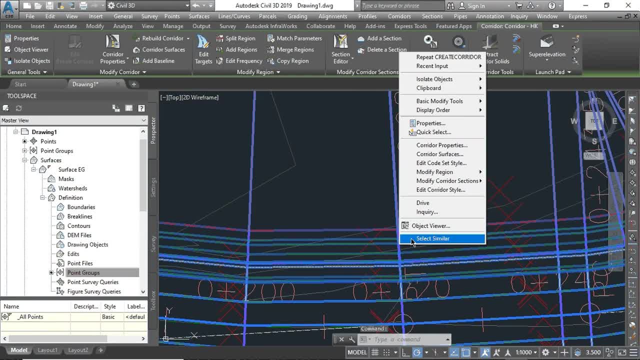 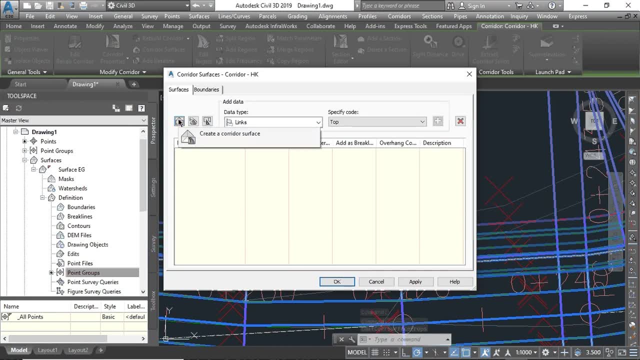 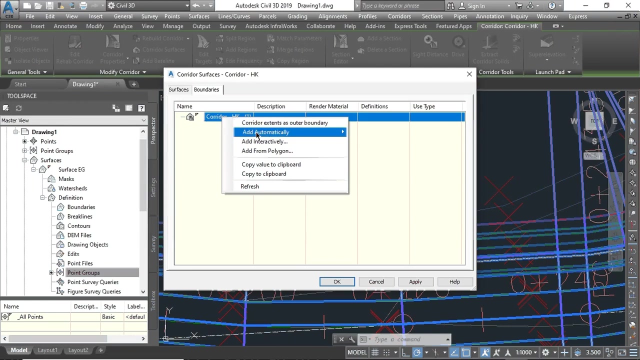 Now we go to the next one To the right we need to go to. I have click and go to corridor surface. you come to home, create a corridor surface, then you add. you tick this window, then you go to boundaries. you right click on corridor, then you add. 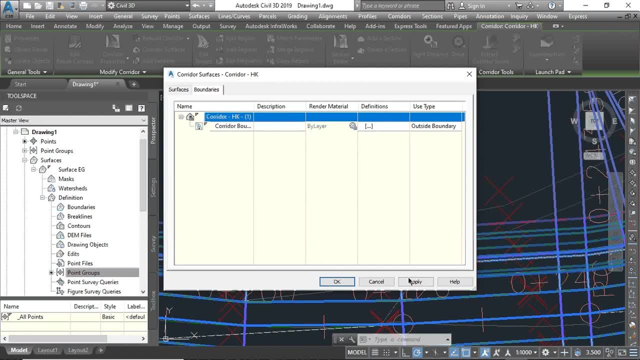 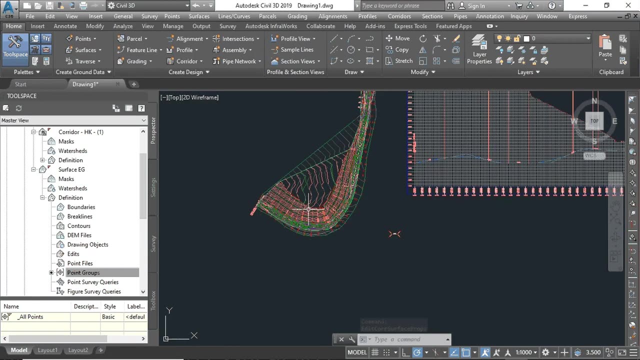 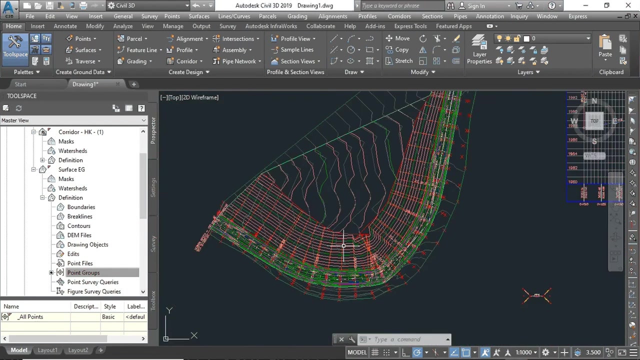 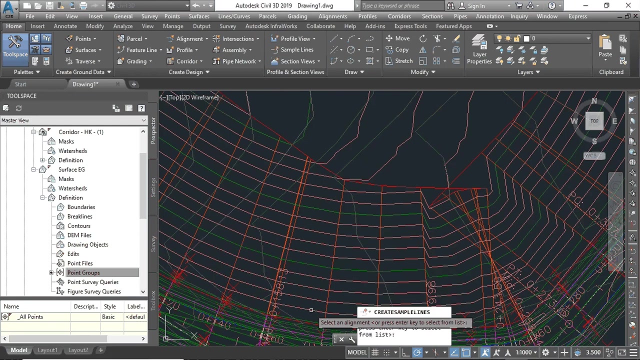 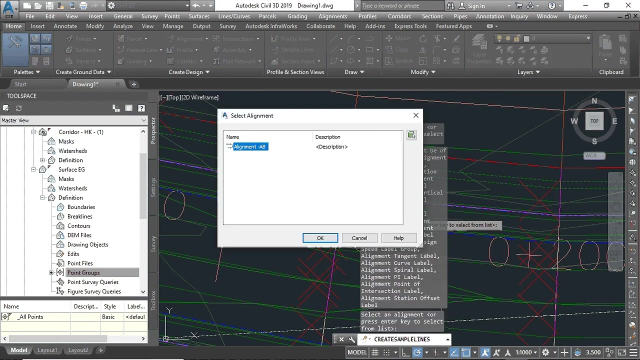 automatically. then click on daylight and you apply. we build the corridor again and okay. after that we go to sample line. we click on sample line. we go to sample line, we click on sample line. we click on sample line. we click on sample line. you zoom and click on this tick line, righty click. then okay. 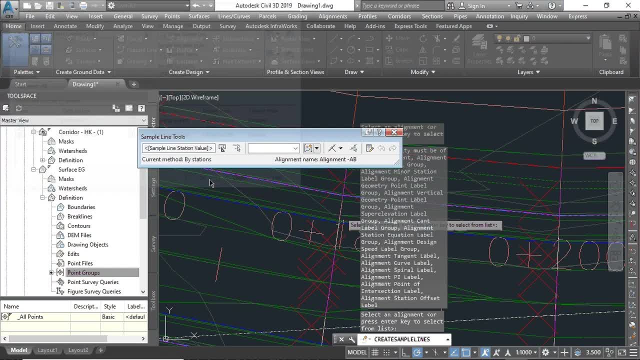 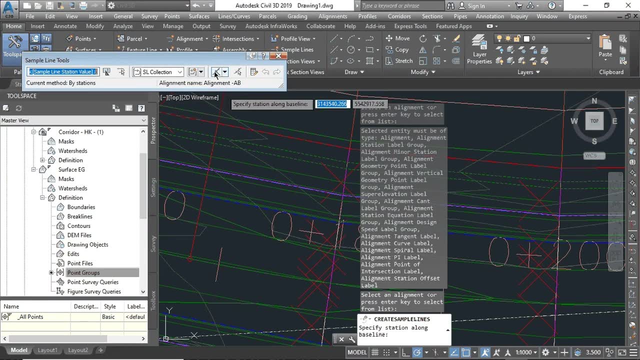 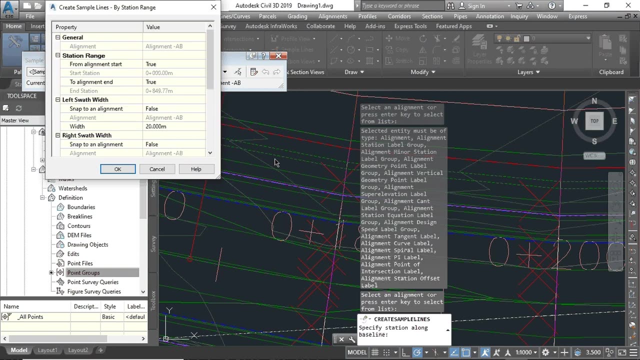 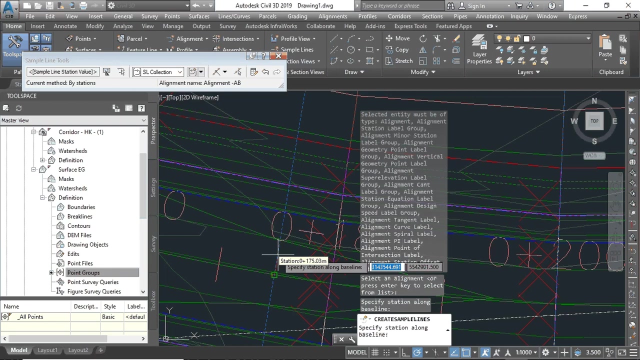 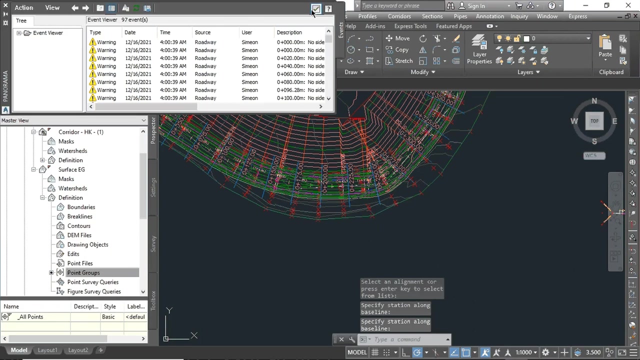 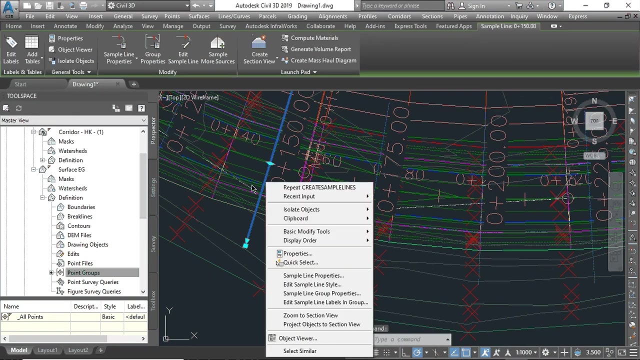 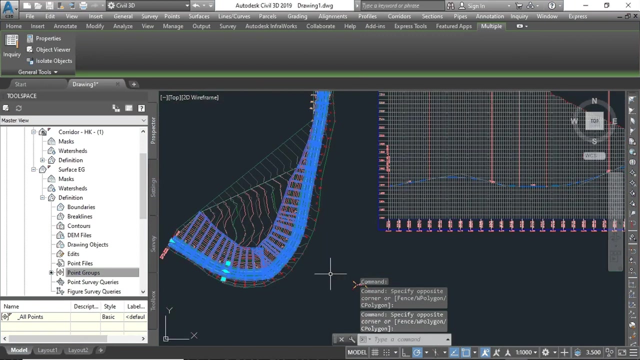 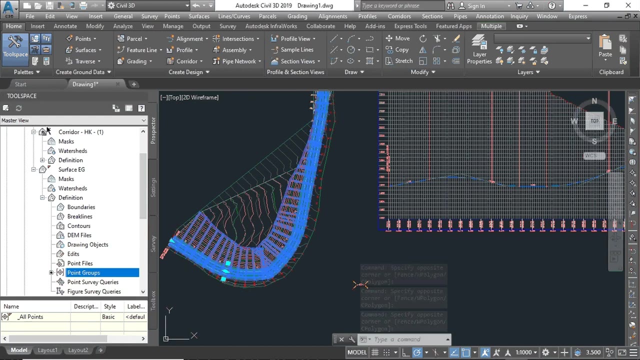 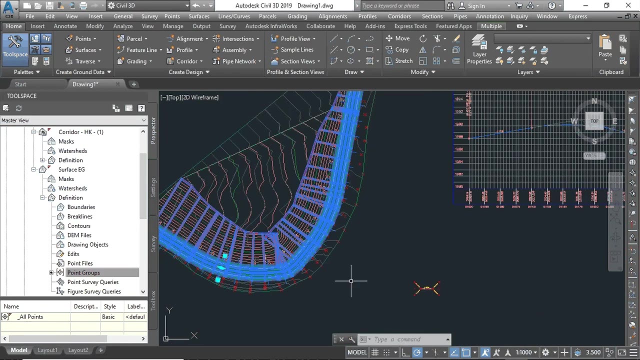 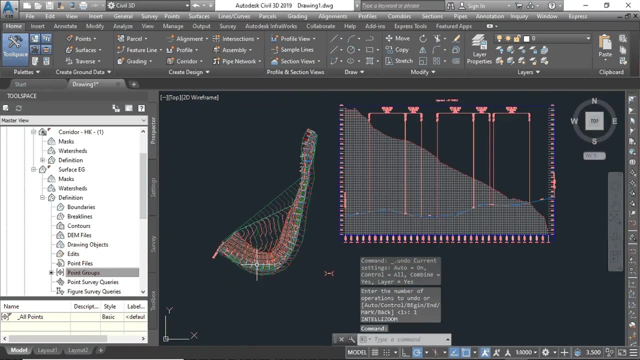 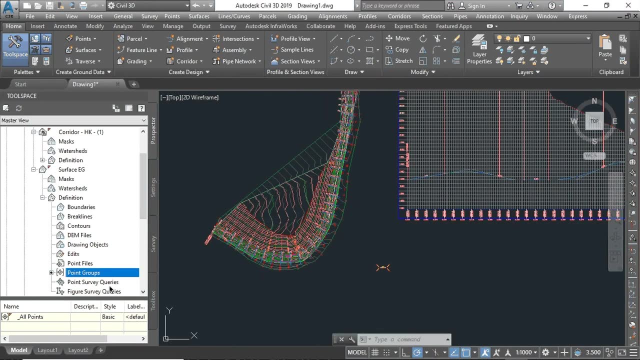 then after that you click okay, you see this toolbar, sample tool, and you choose by range station. you edit as you see you have used 25 interval. then at range end you choose true and okay. so after that you come, We come to home. so we are on home, you, we come to. we are still on prospector, we come. 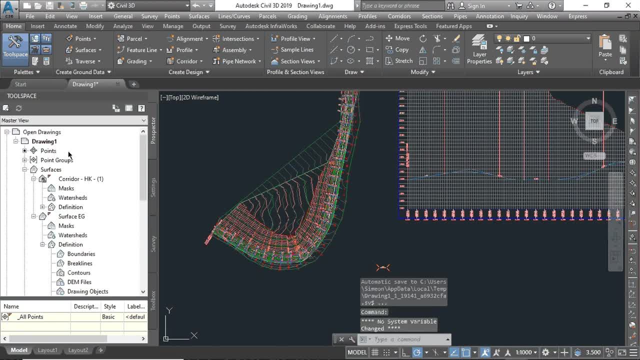 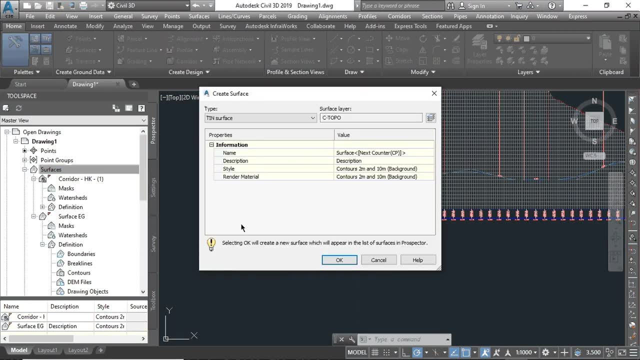 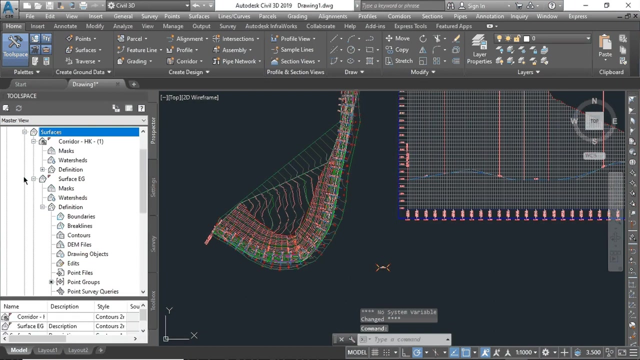 to surface again our surface. then we create another surface. let call it surface2, then you edit our background. let us use 1 and 5, then we click ok, We come to the surface. we have created our surface2, then you click on plus sign. then 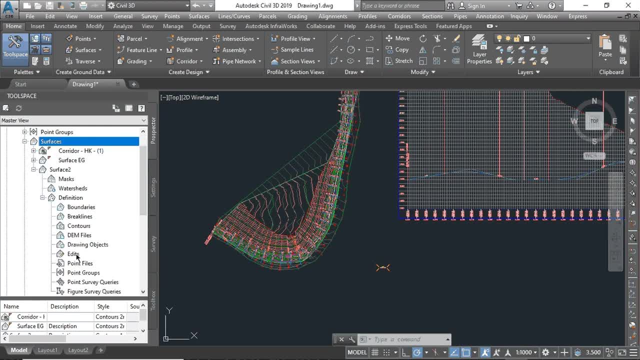 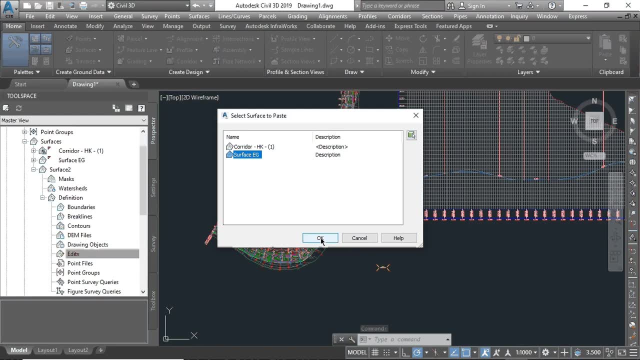 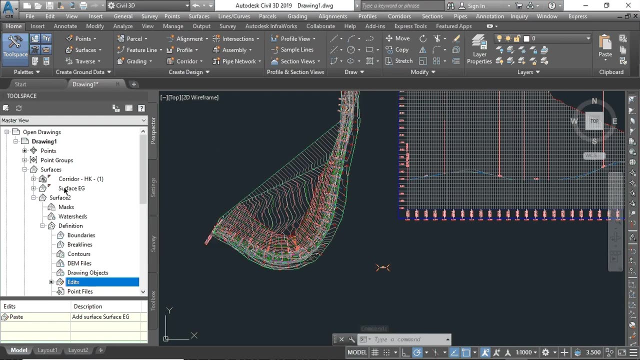 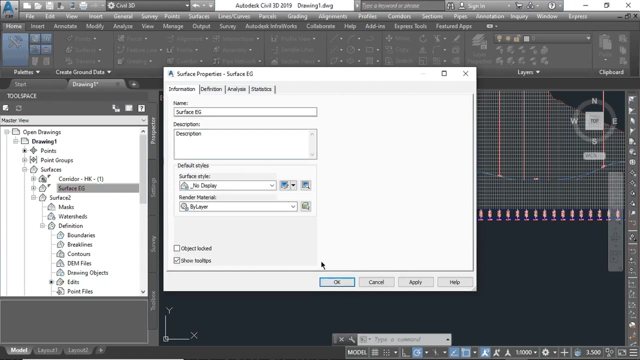 you go to definition, You go to edit, then you paste surface, paste it in surface1.eg, then ok. After that we come to surface1.eg. you right click, then click on surface properties. we come to surface style. we choose no display. 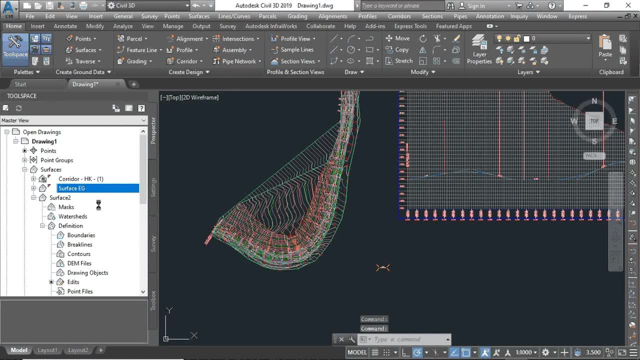 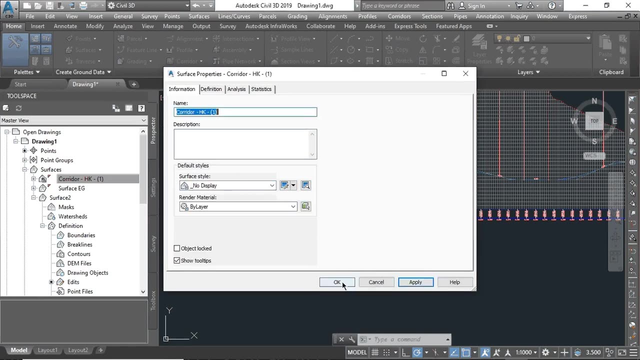 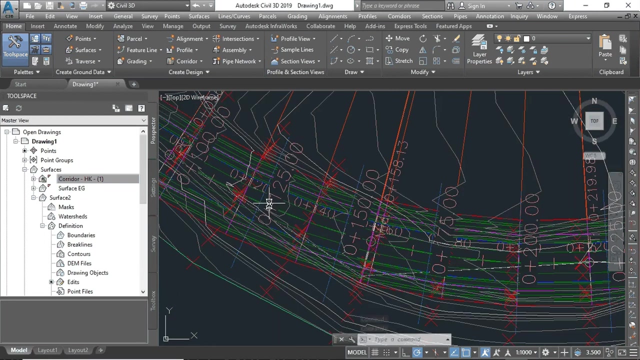 Then you apply ok. Also, do it on corridor. click on corridor, right click on corridor, surface properties. you surface style. choose no display, you apply ok. So by now you should view your surface, Your surface, Ok. 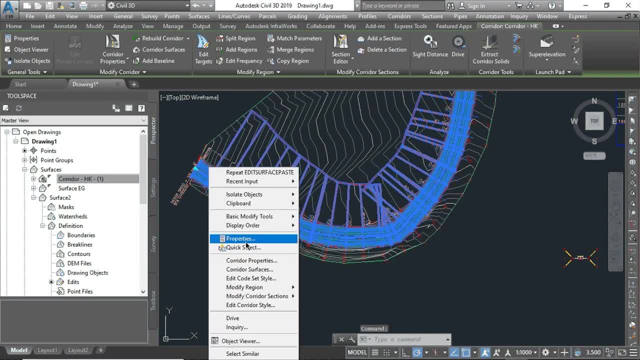 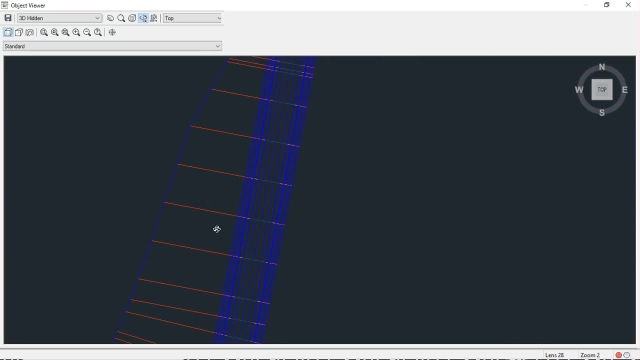 Ok, Now we come to our corridor. Then you right click, you select your corridor. then right click you choose object viewer to see how it look. This is our corridor. Also, you should view a corridor by driving it. 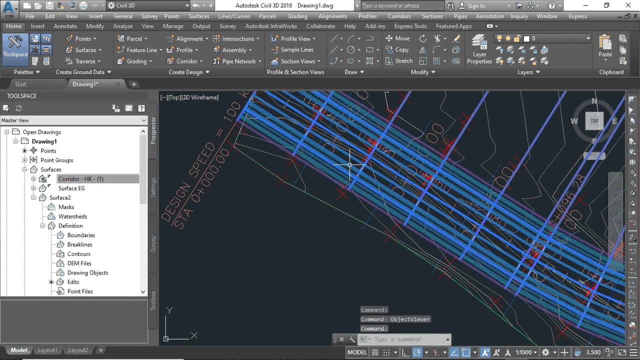 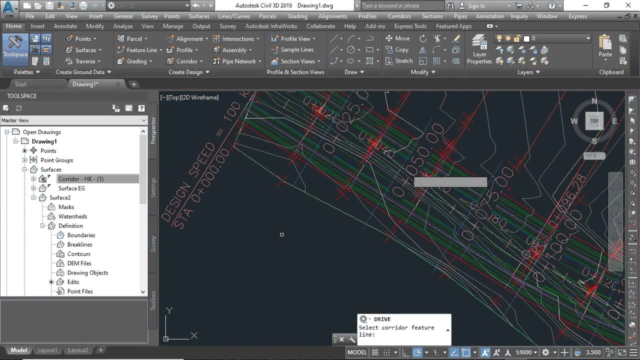 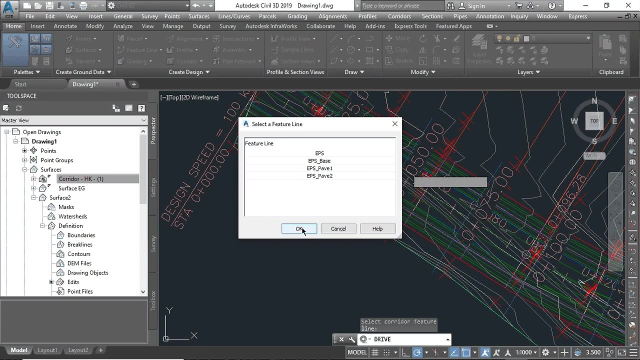 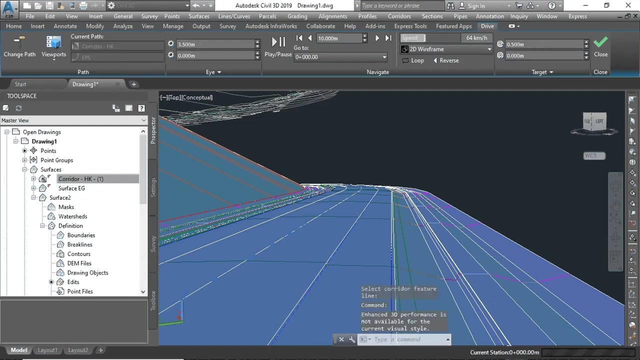 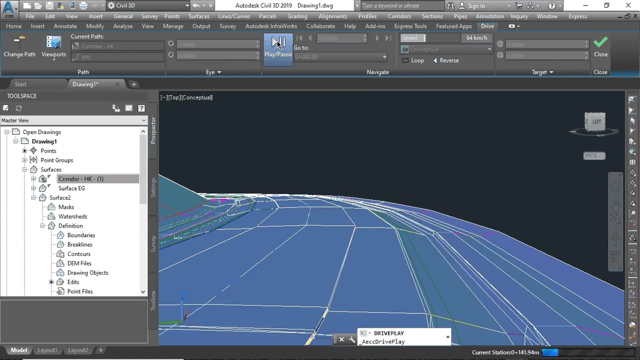 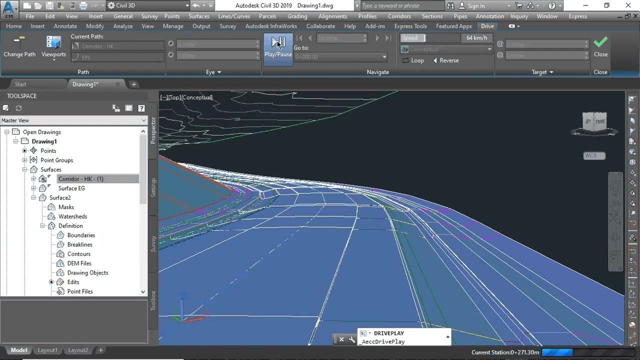 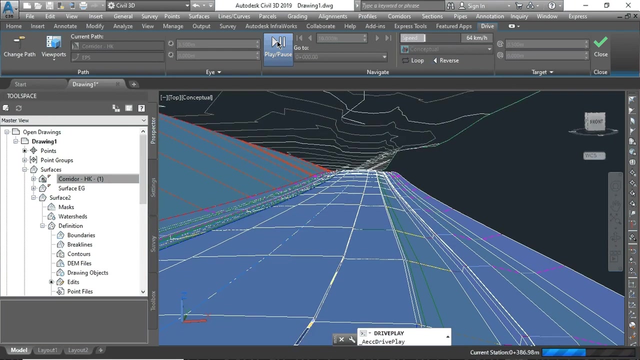 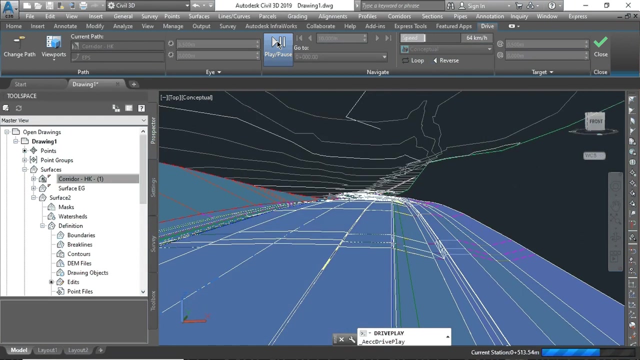 Ok, in motion. you select it. then you click on drive. you see this symbol they gave us. you come and click here. then you choose. okay, as you see, by now we can drive and view our road. this is how it will be look out. is designed as you see. this is our, our load. we designed so you can close and continue. 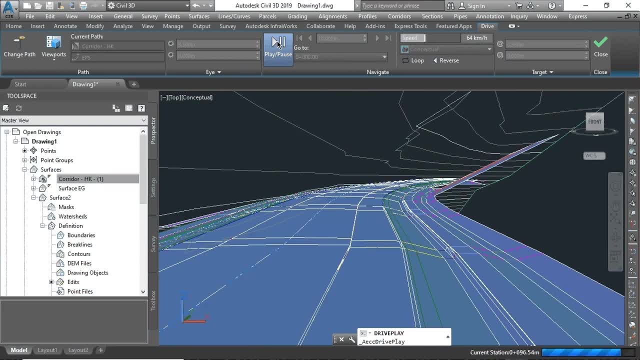 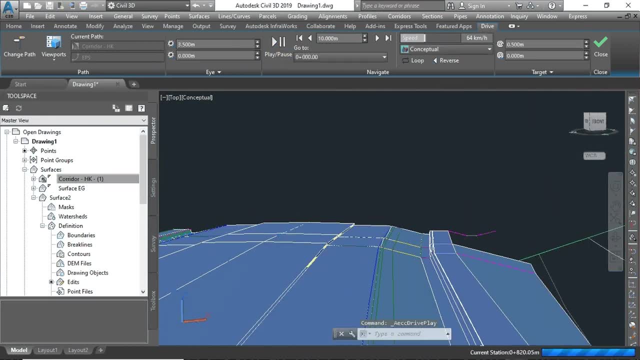 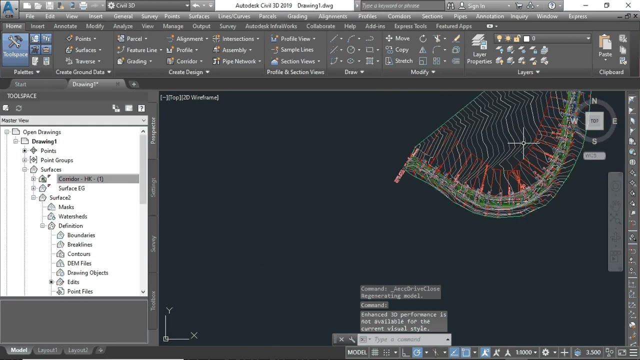 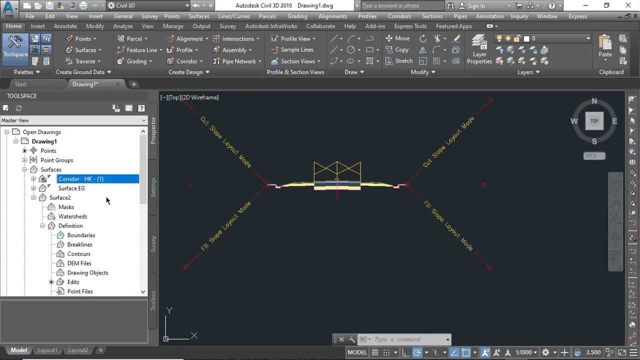 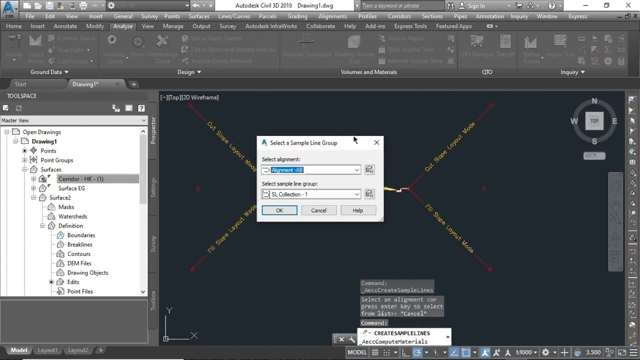 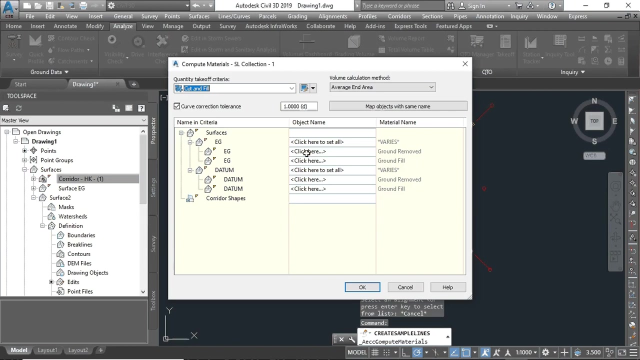 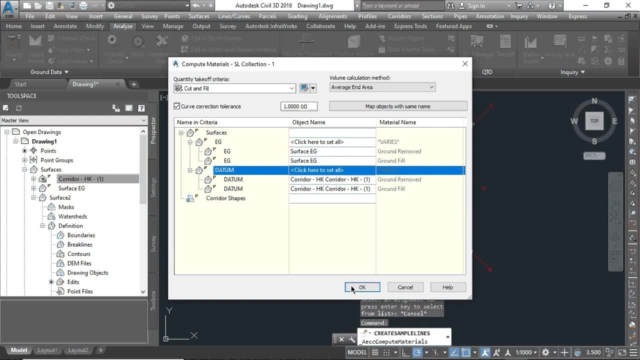 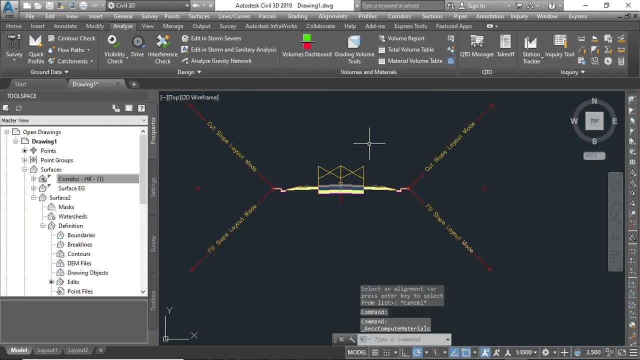 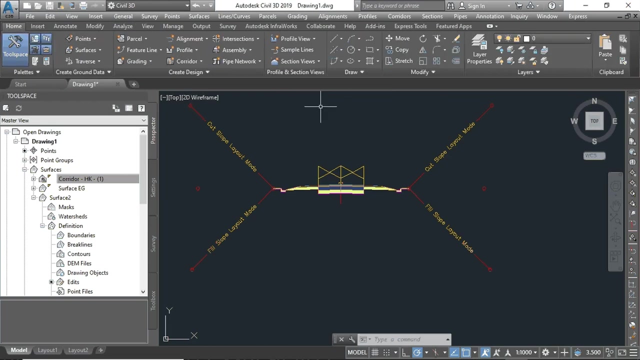 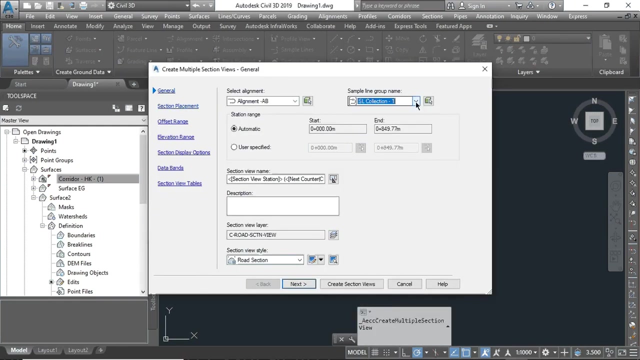 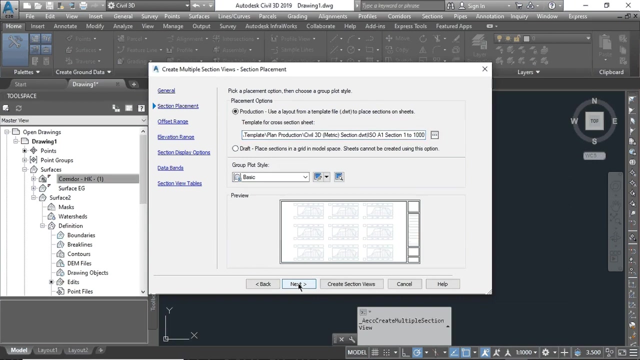 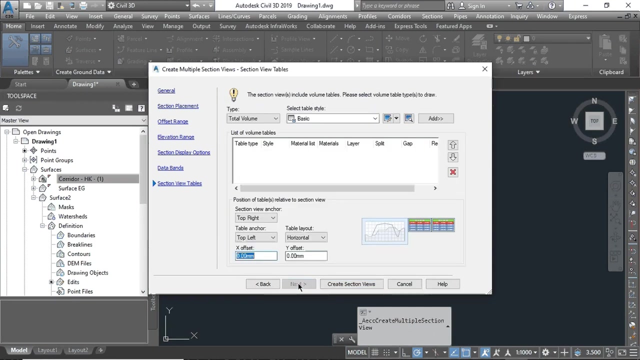 you select corridor, then okay, after clicking on compute material, you come back to home. you go to home, you click on some section views, then create a multiple section view. after that you click next, next, next, next, next, then you click add, then you click create section views and yes. 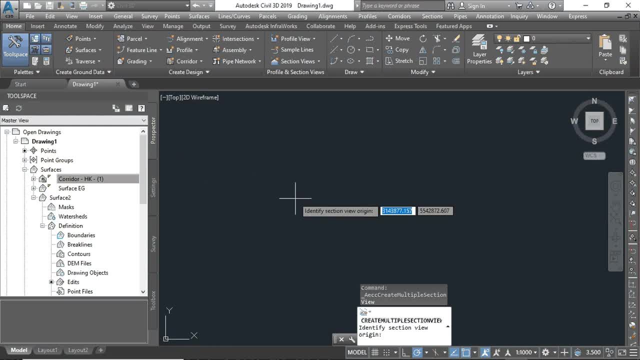 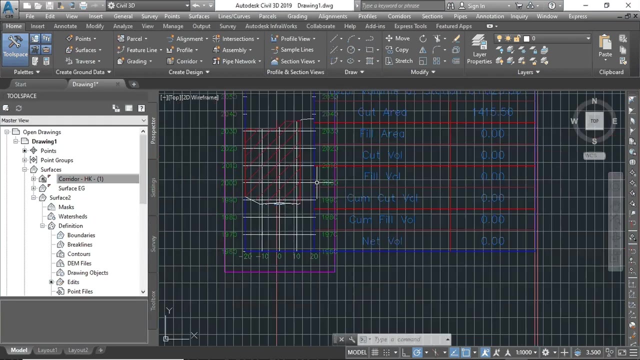 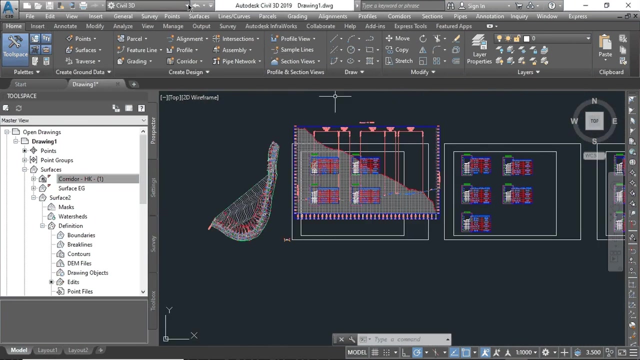 so you come to the window and click where you want to display your, where you want to display your volumes of your quantities. i'm sorry i displayed it in. i displayed it in a bad position, but this is the procedure of how we will display it, how we get quantity or volume and fill and cut. 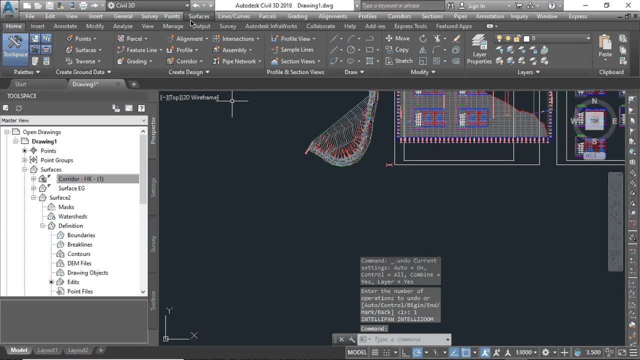 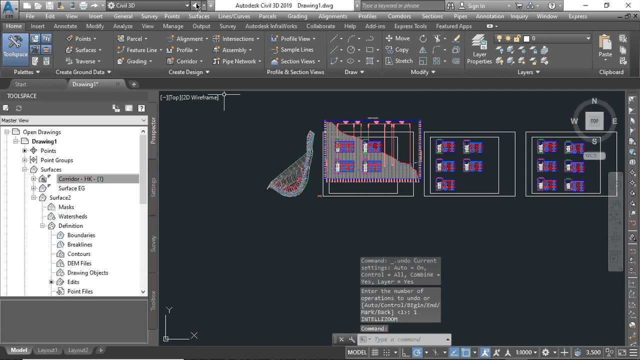 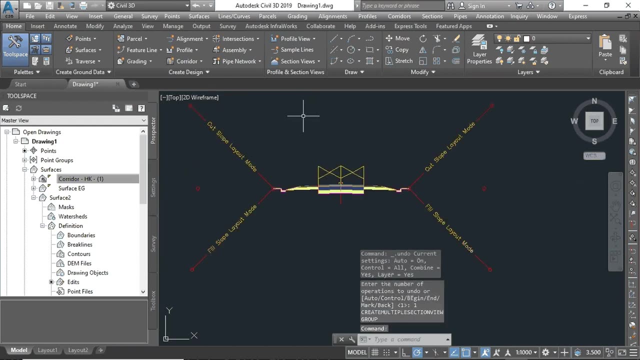 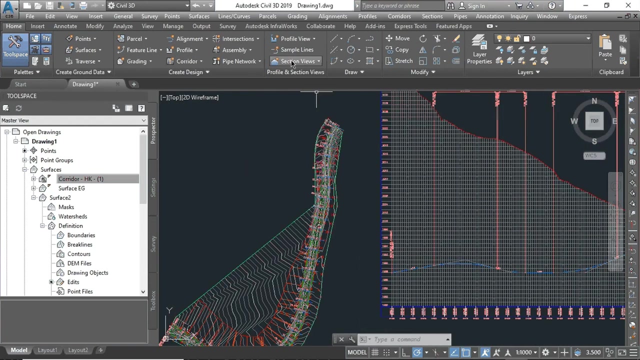 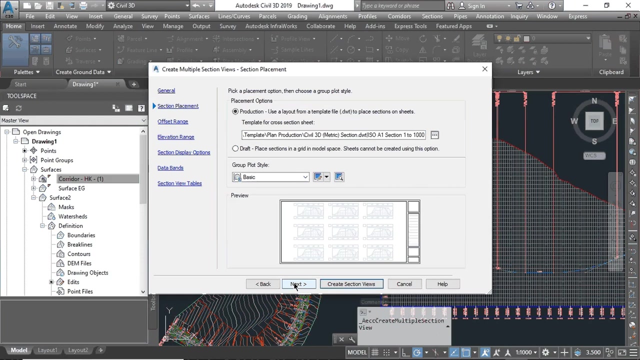 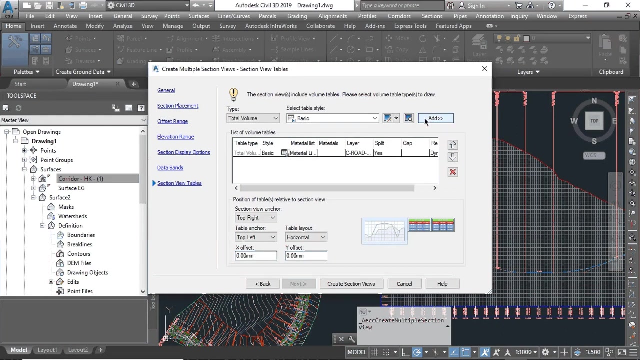 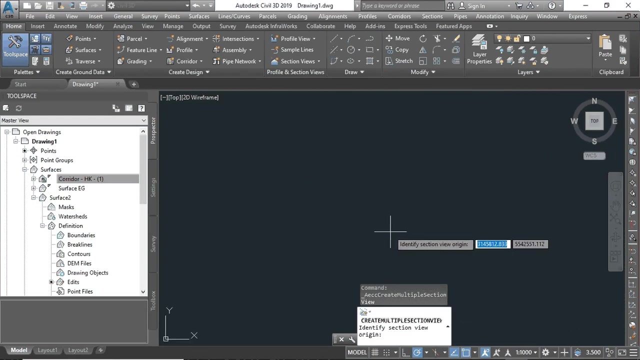 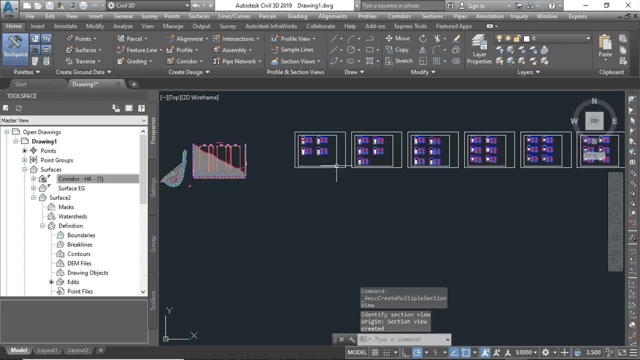 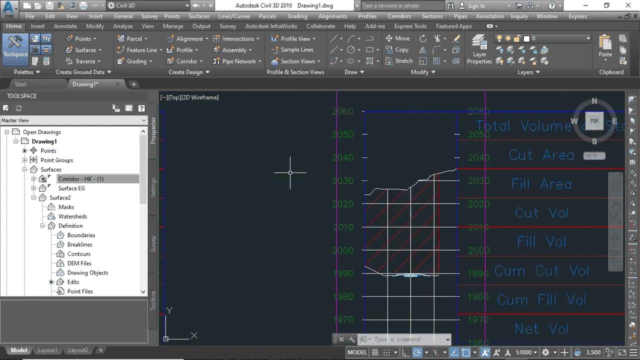 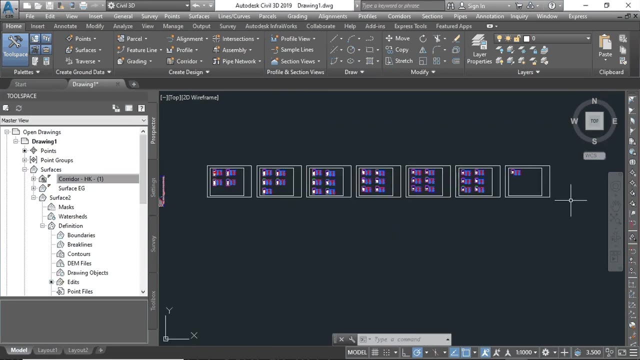 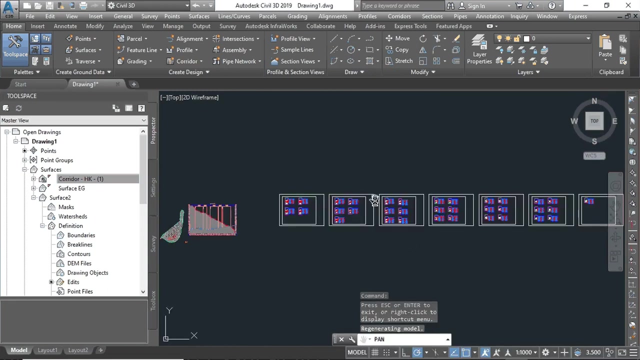 our quantities. this is our quantities: total volume, feel and cut as we see this, and if there are many, you make a zoom, and if there are many, you make a zoom extend. but here there is no, no problem, everything good way. so, after getting our quantities, we are going to see how to generate volume, total volume report. you, you come to home. 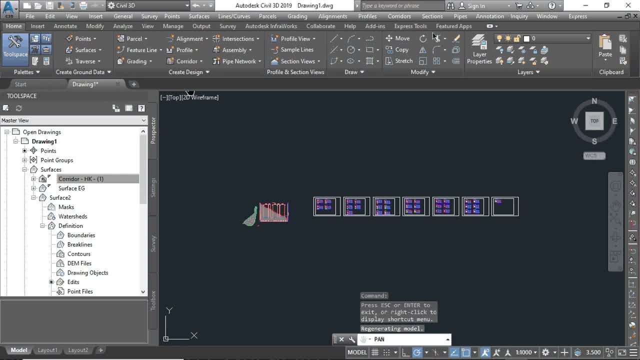 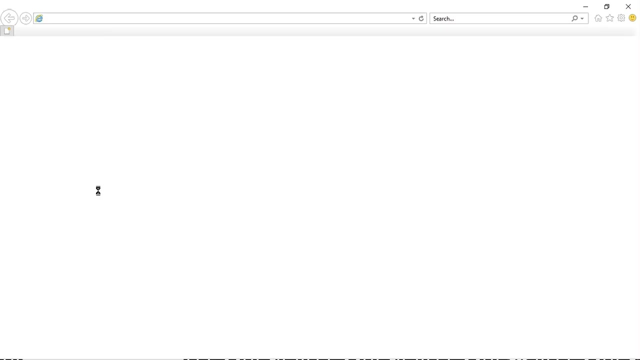 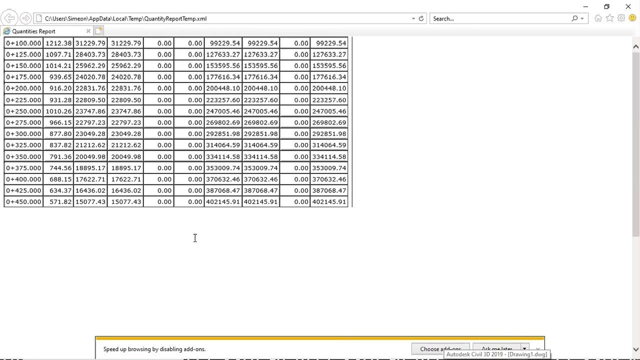 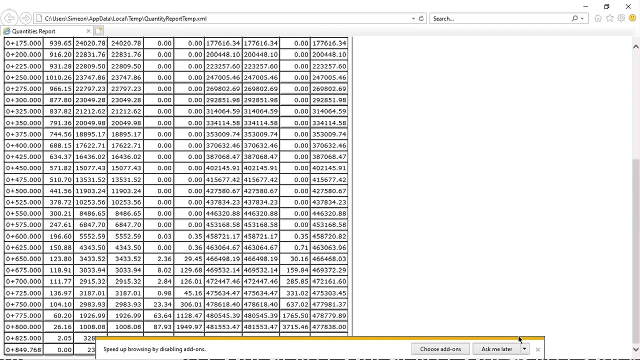 then you, you go to sections, then create generate. after clicking on section, you click on generate volume report. then okay, after clicking ok, you see there is some tool, two bars which are being opened. so it is still loading. as you see, this is our table of, this is our table of. 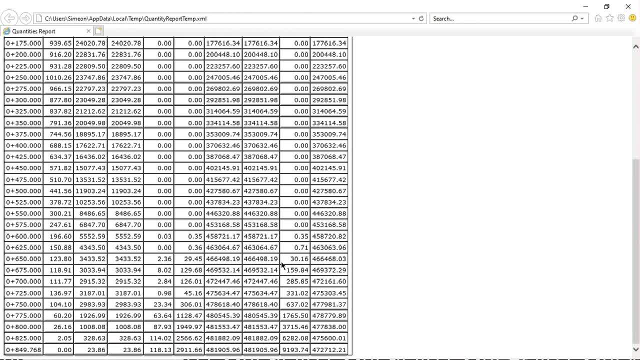 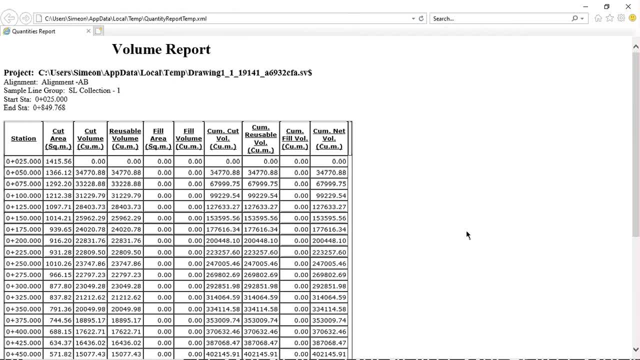 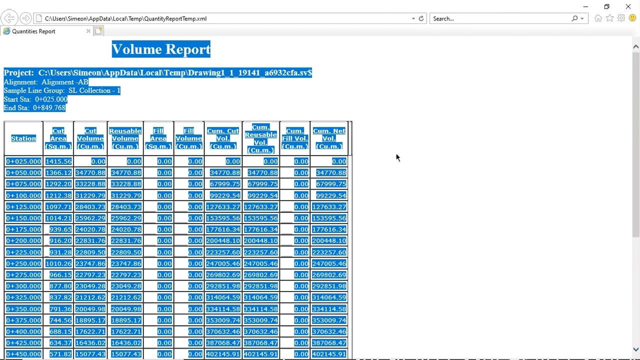 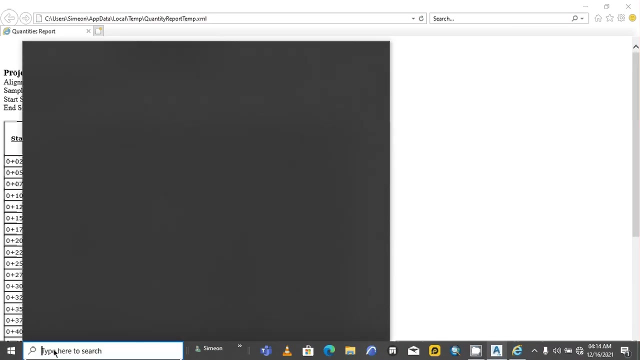 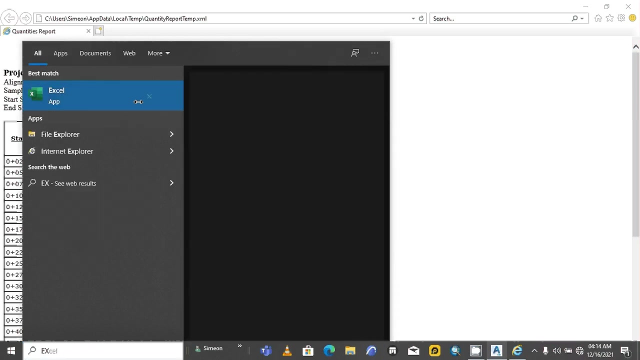 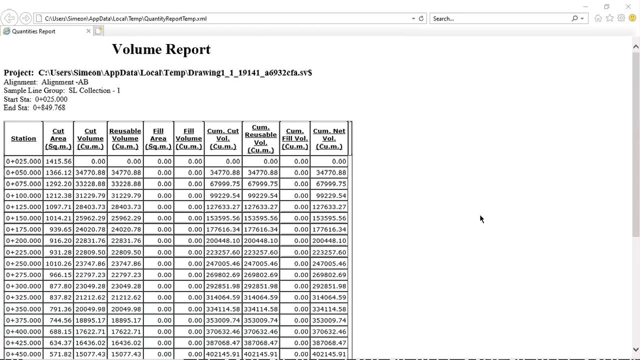 of cut and fill for our project. so after that we we represent this table in in excel. you ctrl plus a to select, to select all, then ctrl plus v, ctrl plus c to copy. then we open our excel. this is our excel notice: the DaVinci Live. 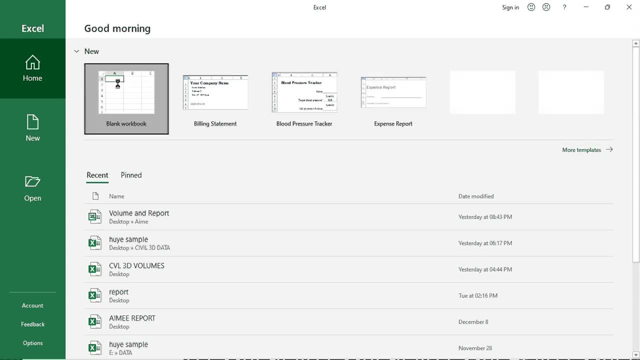 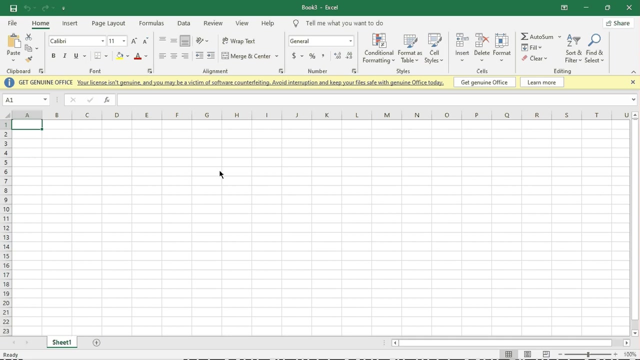 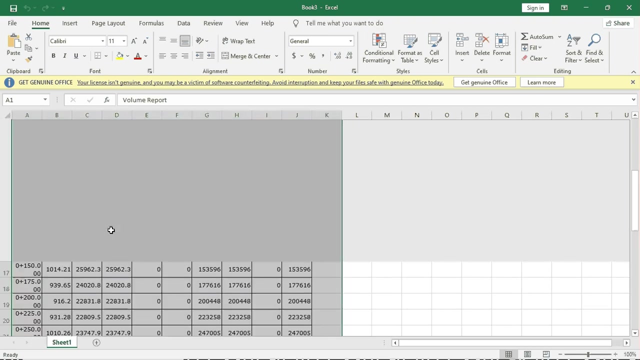 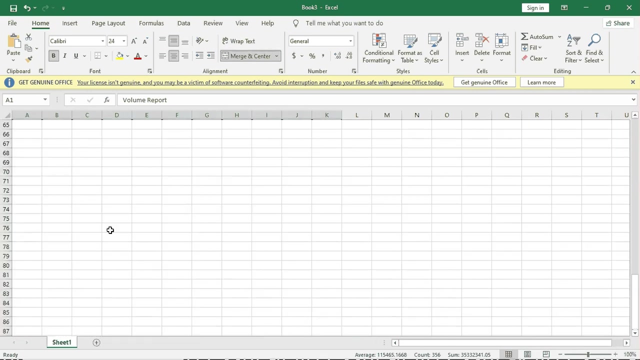 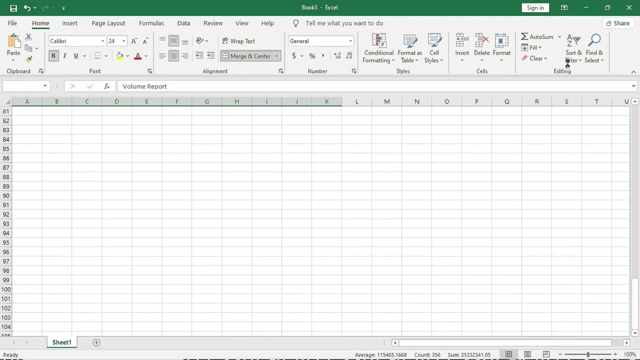 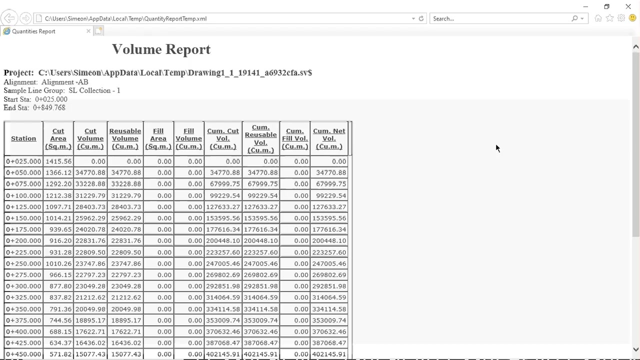 from excel. so then you, if you taste your quantities in this space of Excel, ctrl plus V, then you copy. as you see, this is our, our final report. I think it is not, so. thank you for for your attention and for encouraging me to put any fault in standing this software, third thing, so. 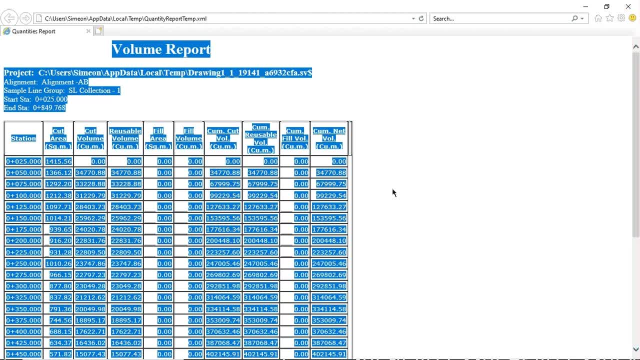 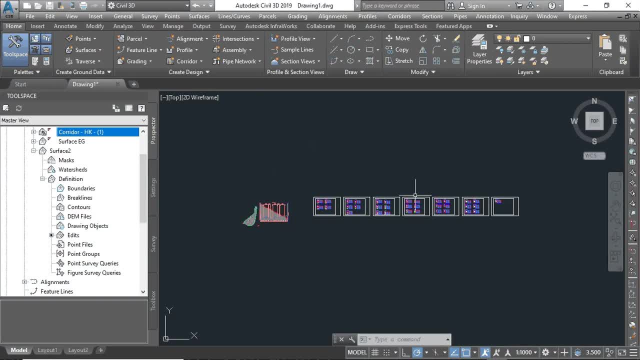 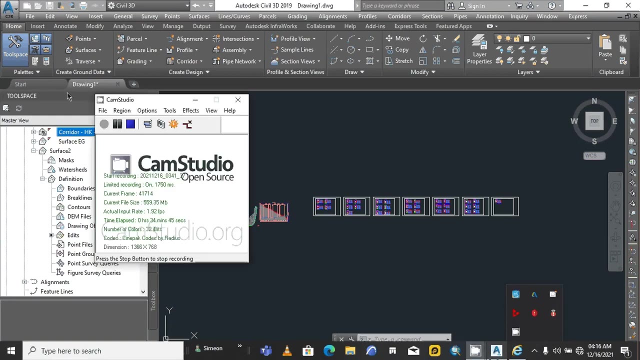 ok, you so much. I think this is my short tutorial to explain how I used to make that assignment of not design. so thank you so much. 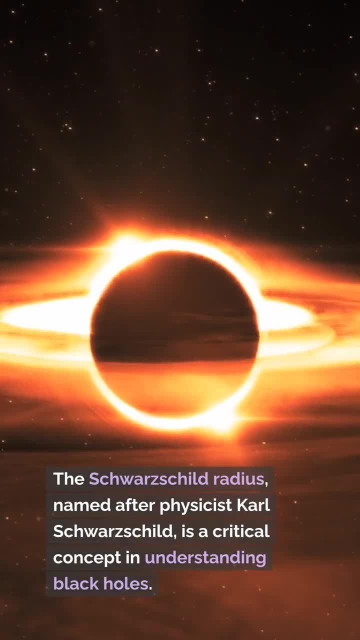 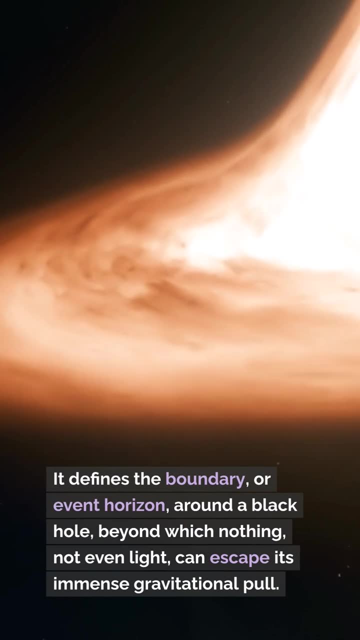 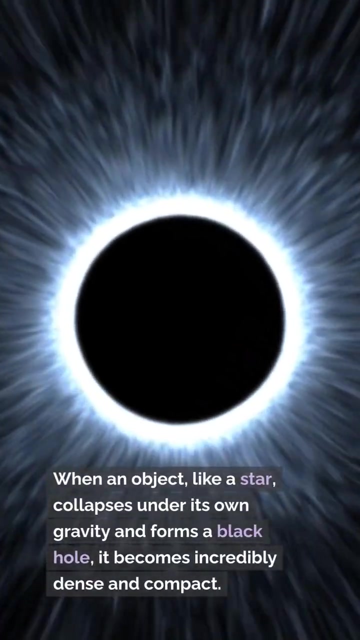 The Schwarzschild radius, named after physicist Karl Schwarzschild, is a critical concept in understanding black holes. It defines the boundary or event horizon around a black hole beyond which nothing, not even light, can escape its immense gravitational pull. When an object like a star collapses under its own gravity and forms a black hole, 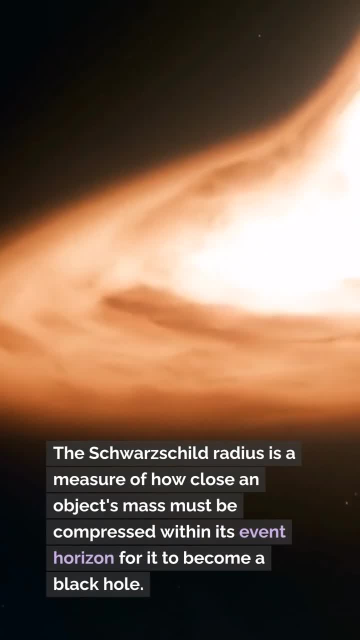 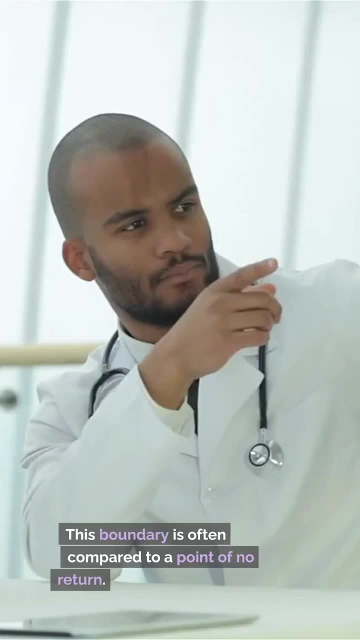 it becomes incredibly dense and compact. The Schwarzschild radius is a measure of how close an object's mass must be compressed within its event horizon for it to become a black hole. This boundary is often compared to a point of no return. Anything crossing this boundary is 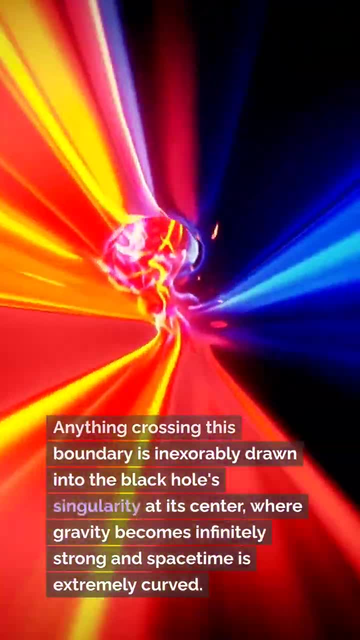 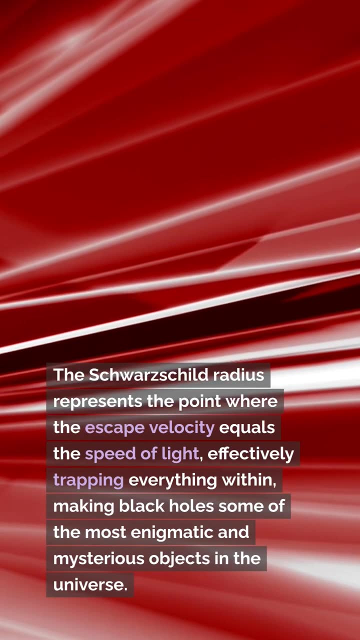 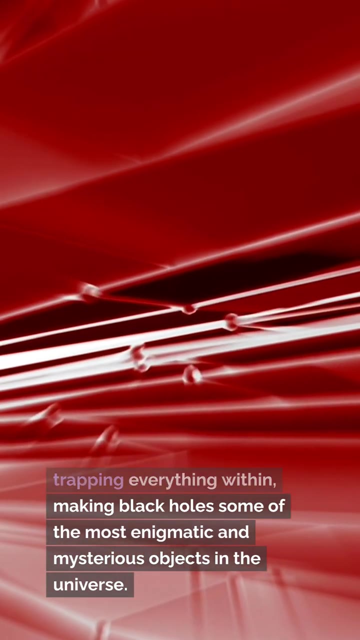 inexorably drawn into the black hole's singularity at its center, where gravity becomes infinitely strong and space-time is extremely curved. The Schwarzschild radius represents the point where the escape velocity equals the speed of light, effectively trapping everything within, making black holes some of the most enigmatic and mysterious objects in